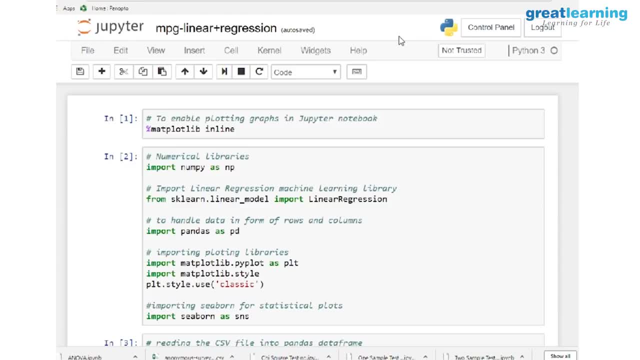 MPG, linear regression. It is like your hash bang in Java programs, where it is giving instruction to the compiler. Here we are giving instruction to the Jupiters that plot your diagrams in the notebook. If you don't give this line, your diagrams will not be part of your notebook. 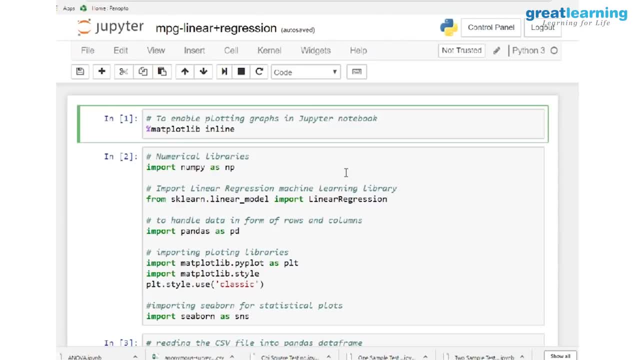 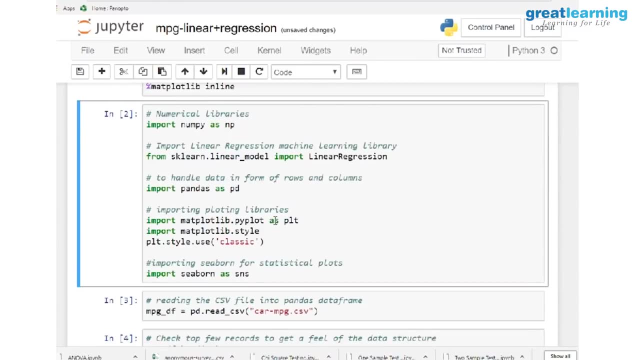 That's all it is. So go ahead and execute this. I am importing all these libraries which I need: numerical Python as NP. Import NumPy as NP. This is a standard practice to always represent this package as NP, But it doesn't have to be. You can simply say: import NumPy From scikit-learn package. 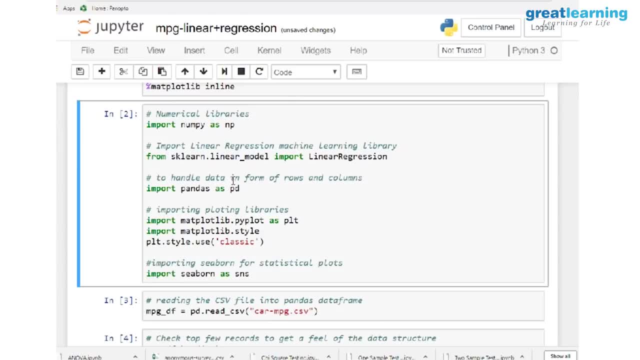 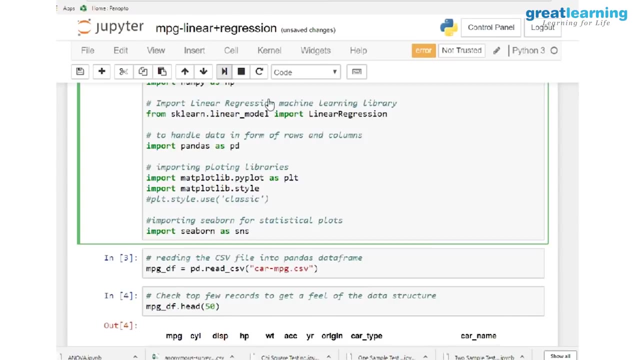 I am importing this linear model. There are different types of linear models. I am importing linear regression, Then Pandas as PD, Matplotlib as PLT. I am going to use Seaborn libraries wherever I need to plot. I am biased towards Seaborn, so I am importing Seaborn SSNS Go. 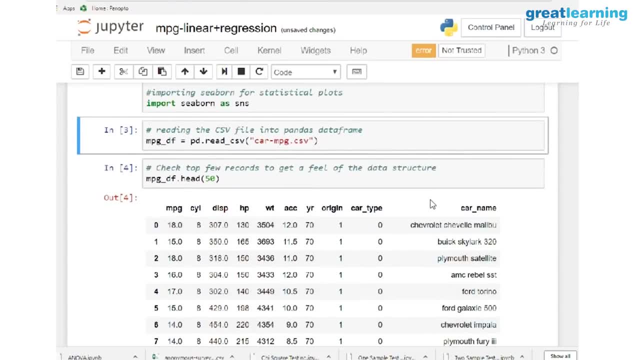 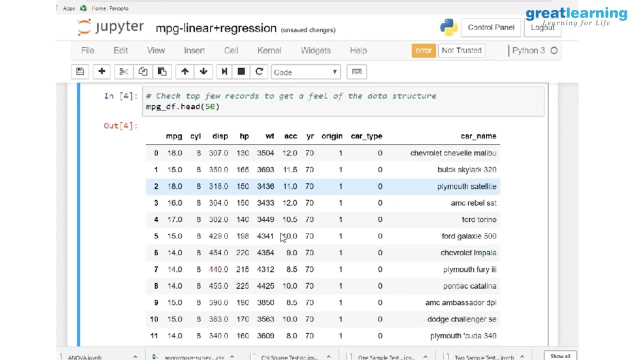 ahead and execute all this, We are going to read a file called, let's say, car-mpgcsv. Once again, I assume a lot of people ask me: do these files have to be CSV files? The answer is no. The file can be an RDBMS data set. It can be a NoSQL data set. 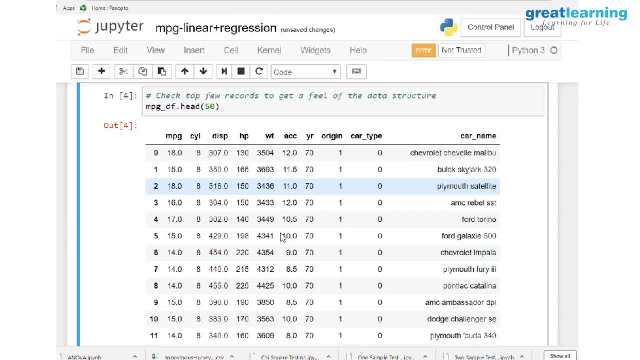 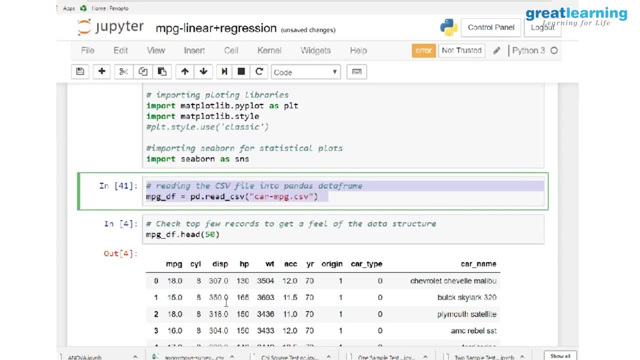 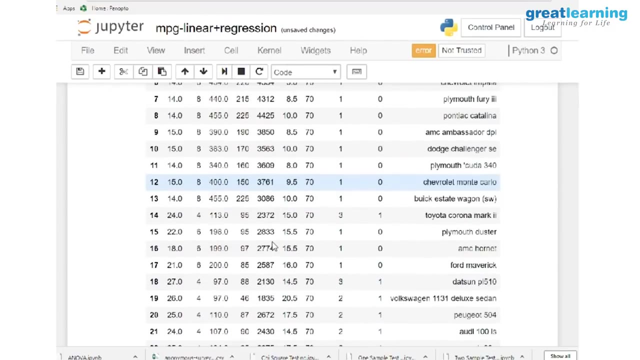 It can be a Hadoop data set. It can be a website also, But we are using csv. If you are able to do this, execute this. Done mpd-head. This is also done Coming down here. you see, car name is car underscore name, You please? 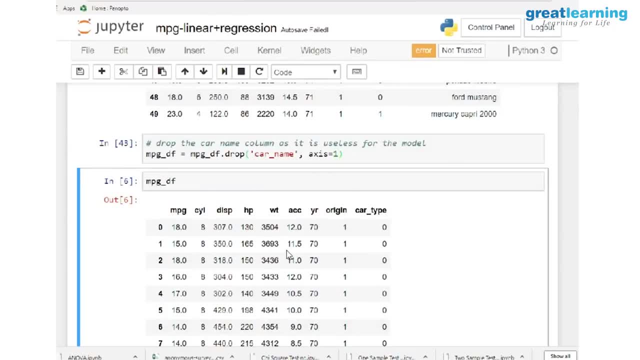 replace this car hyphen name with car underscore name. You may say that by looking at car name I can guess the miles per gallon Japanese car give higher miles per gallon than American cars. You can say that, But then how strong? 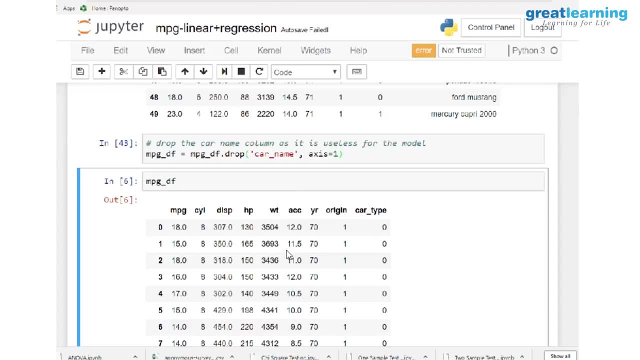 a predictor the car name is of mileage. For example, if the car name is Honda Within Within Honda, there are so many variants with different mileages. Within Toyota, there are so many variants with different mileages right. Hence the car name per se is not a very strong predictor. 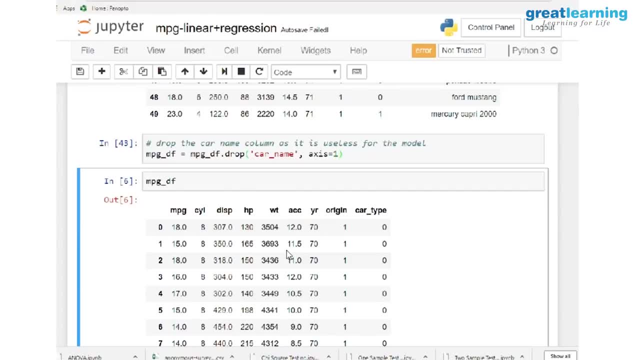 The analysis will also show you that. So I have taken the liberty of dropping the car names. It is not mandatory. It is based on the observation that I have taken the decision to drop the car names because it is not a strong predictor. 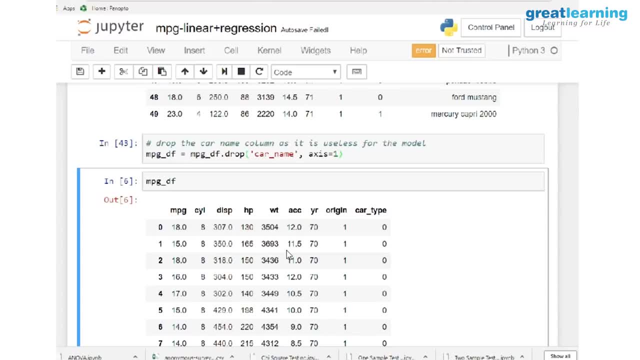 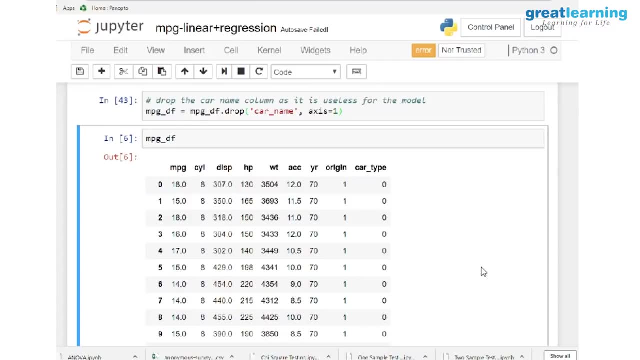 If I had individual car names with model number and all these things, I could have considered that for my model. So next time when you see this mpg underscore df, the data frame, you will see that columns except for car name. In my case I have car type also. 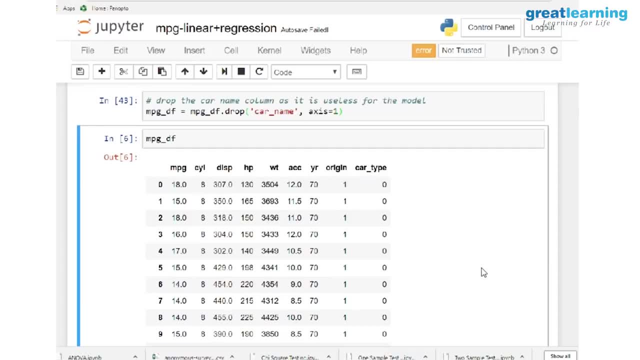 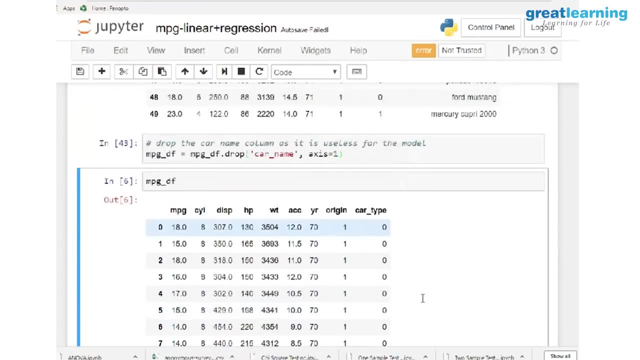 Car type is manual or automatic, Two types. You do not have that data set. Do not worry about that part. Let us move on. You will see that there is an origin column. There is an origin column. Whenever you do these projects, always go to the UCI source: UCI data set. 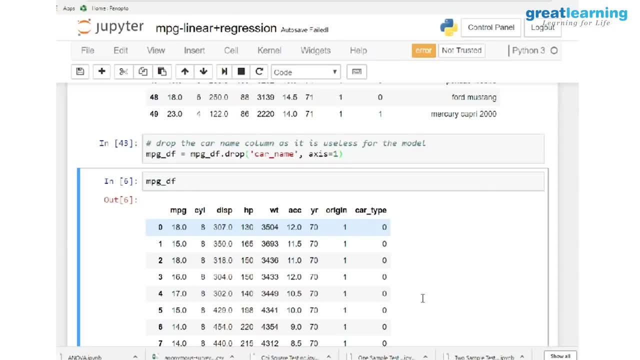 They have given you explanation about each and every column, What these columns are. Today, I am telling you what these columns are. Whenever you come across data sets like this and you have short forms, do not assume you know what it means. For example, there is another data set over there related to cars, where the column name is mileage. 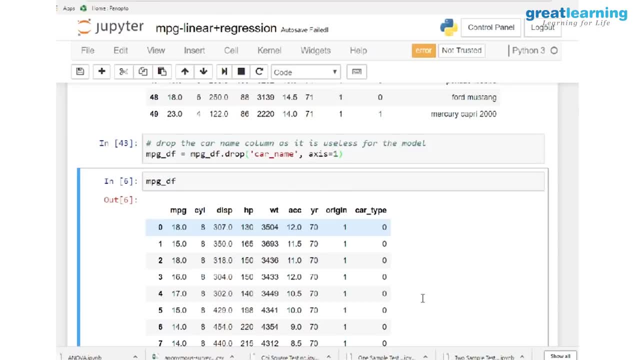 Whereas mileage in western countries means how many kilometers on the odometer. So we should not assume that we know what it stands for. So, whenever you get data, always if you get data like this, Short forms, always make sure you go and understand what these things are. 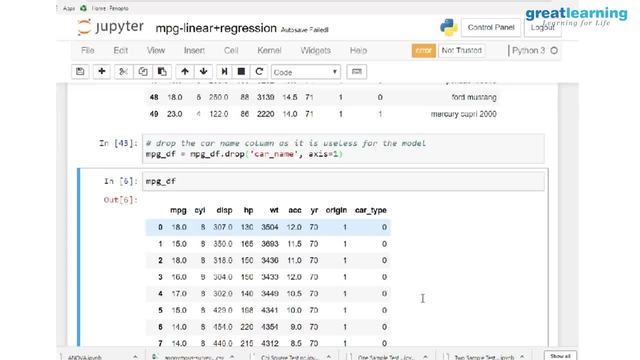 Right now, mpg means miles per gallon And the other thing is origin. What is this origin? This origin is a categorical variable. One means America. America means the American continent. Two means Europe. Three means Asia. In linear models. you cannot use these columns as it is. 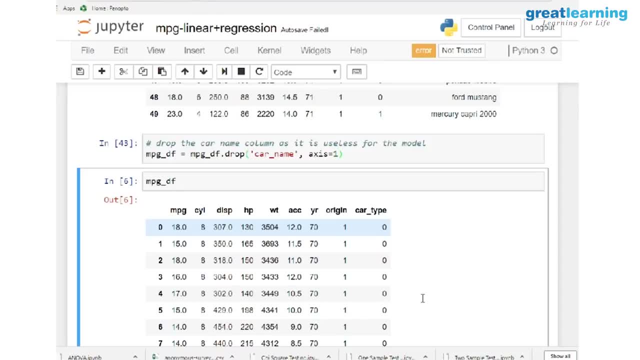 If you use this column as it is, it is a numerical column with 0,, 1, 2.. The algorithm will think that 0 is less than 1 is less than 2.. It will give an order to this, But there is no order here. 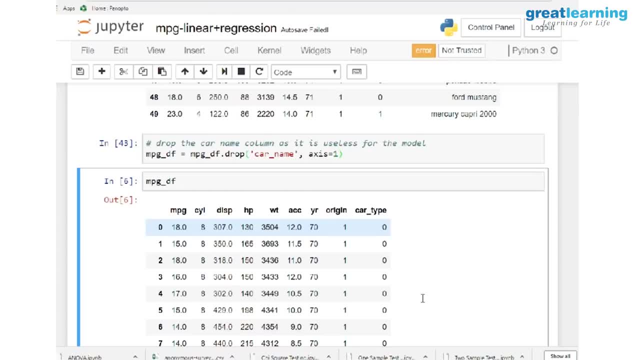 So whenever you come across this column, this kind of columns in your data set, where the values are labels but they are numerical labels, you have to be careful, Otherwise the models will go wrong. What we do here is we convert them into categorical variables. 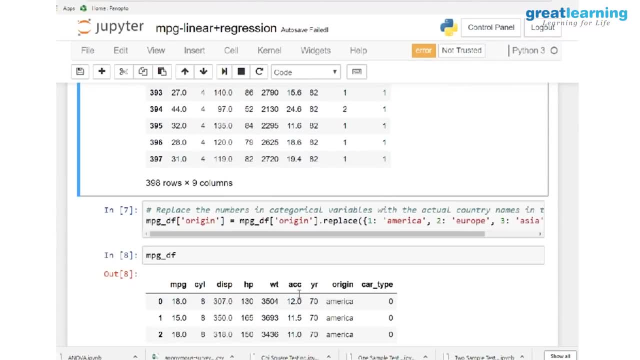 How do you do that? Simple, come down, scroll down, Replacing origin. What I am saying is, whenever you come to America, 1, replace with America, 2, replace with Europe, 3, with Asia. How do I know? 1 is America. 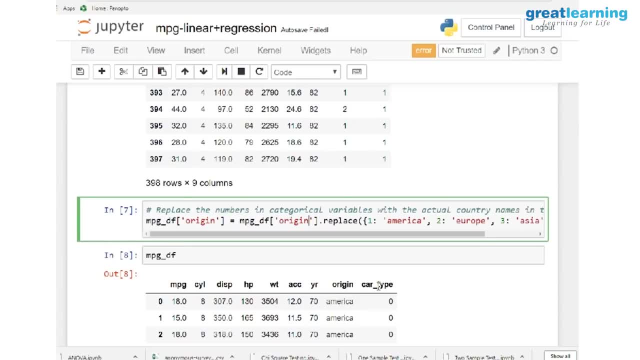 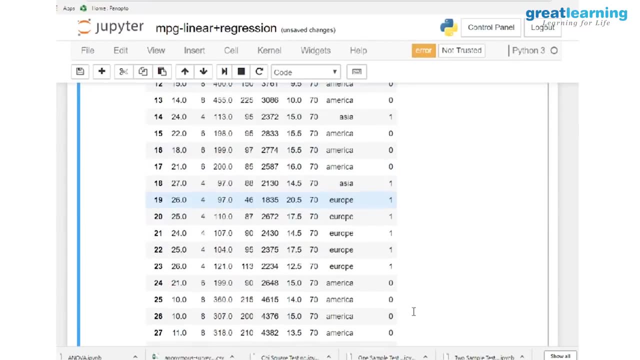 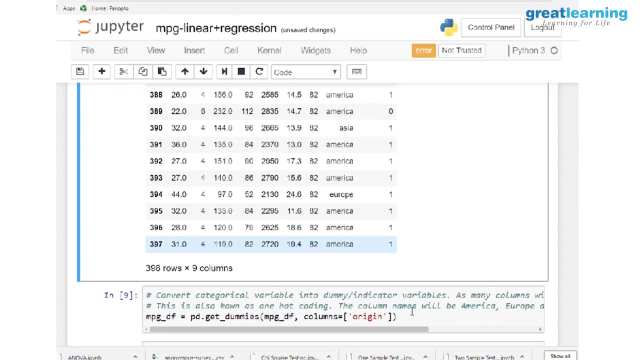 I have gone and read about this data set And they have explained what this 0,, 1,, 2 is. So I am replacing that over here And you will see that origin is replaced with the appropriate continent names. But you cannot use strings in your model building linear models. 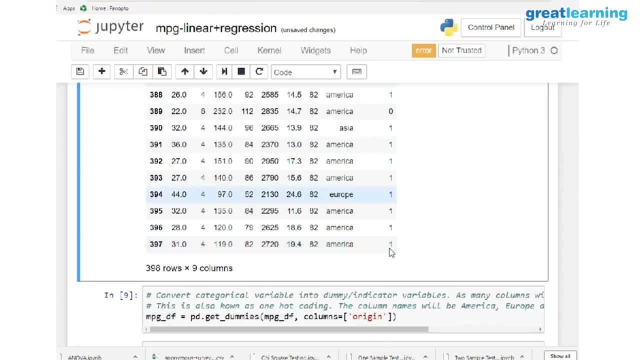 We cannot use strings in linear models. We have to convert them into numbers. To convert them into numbers, what we do is we convert into what is called 1, 1.. We convert them into what is called 1-hot coding. How do you 1-hot coding? 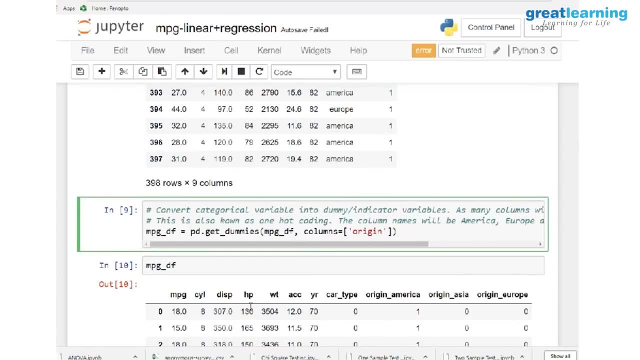 Simple From pandas I call a function called get dummies. This function creates all the 1-hot coding for me. What I am saying is get dummies and run this dummies operation on this data frame and the column called origin As a result of it. what it does is it drops the column origin and replaces with these columns. 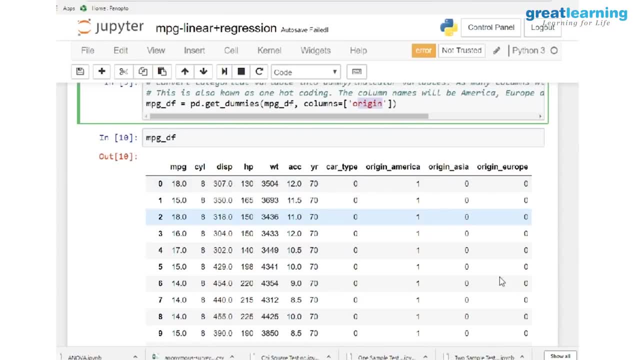 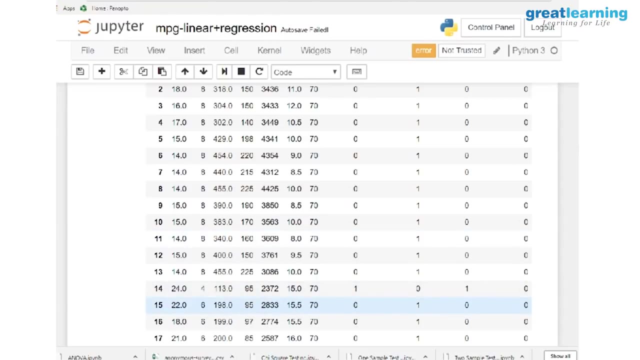 Origin America: origin Asia. origin Europe. All the cars which are manufactured in America will have 1s in the origin America column, will have 0s in other columns. All the cars which are manufactured in Europe will have 1s in the Europe column and 0s in the other 2 columns. 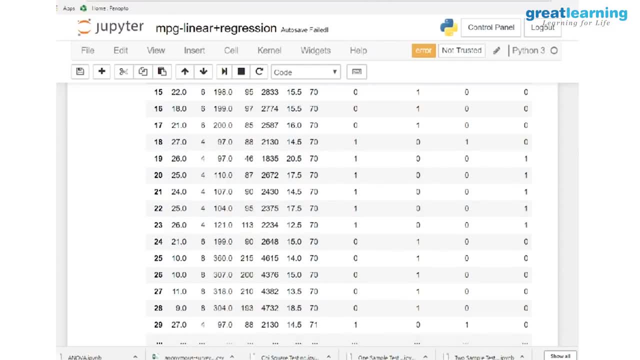 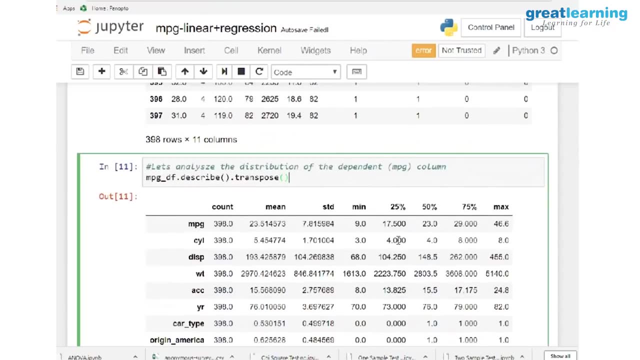 All the cars which are manufactured in Asia will have 1s in the Asia column and others will be 0s. This is called 1-hot coding. Ok, let us move on. This is a very important step in your analysis, which is basic statistics. 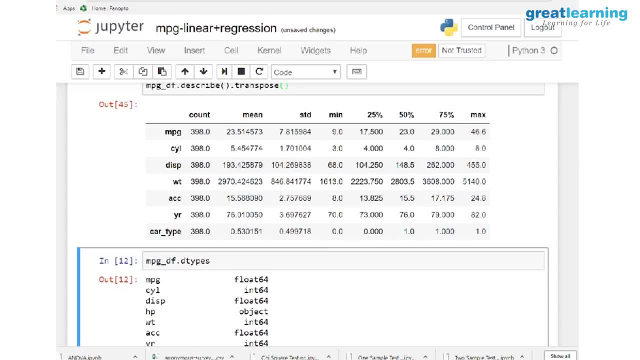 Descriptive statistics, we call it. So we are running descriptive statistics on the columns. Take any particular column. say, for example, displacement. Look at the displacement. What is the mean of displacement? What is the mean? Let us forget the fractions. Look at this. 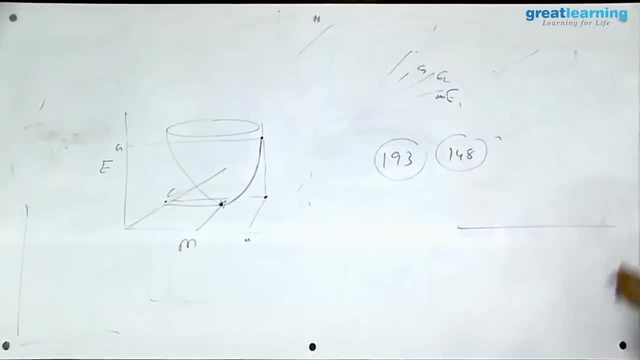 Whenever mean and median are not same, that means you have a skew in your data And mean is on the higher side of median. That shows that you have probably a long tail on the right side. It is a right skew. So if this is my 148, my mean is this 193.. 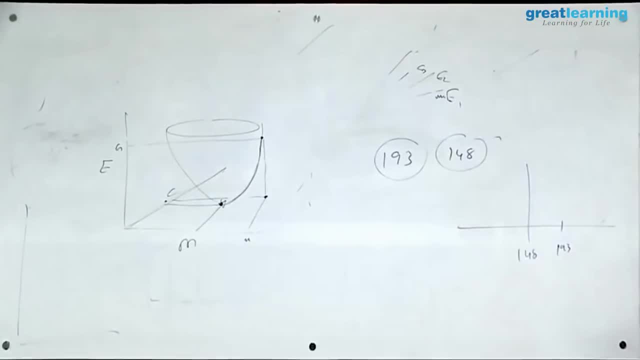 Then looks like my. ok, let us look at further things. What is the distance between your minimum and the first quartile for displacement? Minimum is 68,. first quartile is: So if this is minimum, this is Q1, the distance is around 44.. 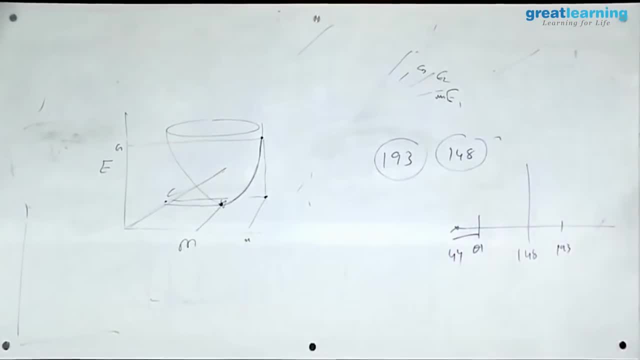 What is the distance between Q3 and max Around? 190 something right Now. look at the tail on the right hand side. It is 190 times And look tail on the left hand side is not even half of this. So that indicates to you your data is badly skewed on the right side. 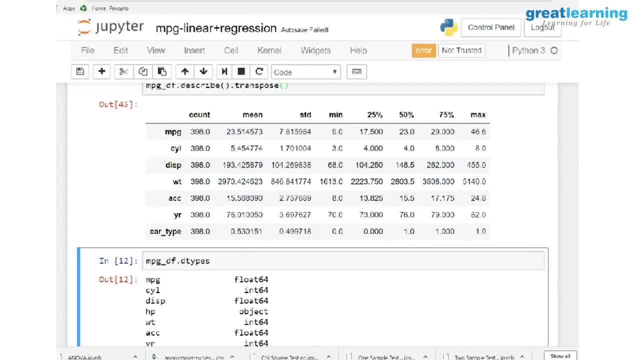 When data is badly skewed on one particular side, or both the sides, you have to go and see: are there outliers which are pulling your mean towards? Mean is very easily impacted by outliers. Are there outliers which is pulling your mean away from the median? 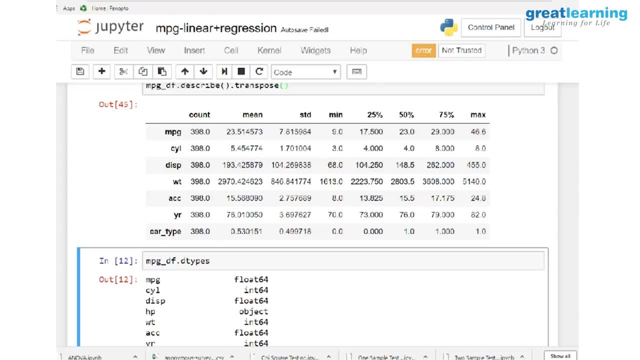 Outliers will bring your models to the knees Right. So this analysis helps you to find which side is the median, Which side is the outlier likely to be And what is the outlier. Any data point which lies 1.5 times IQR interquartile range. 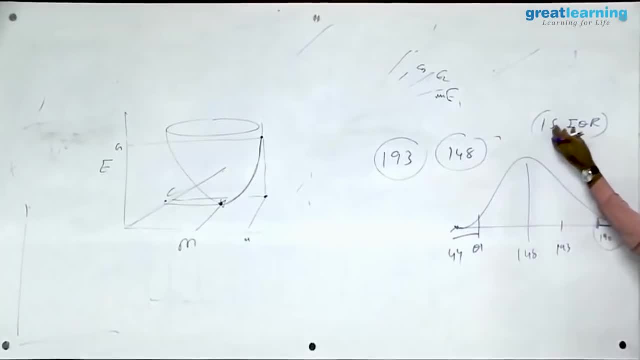 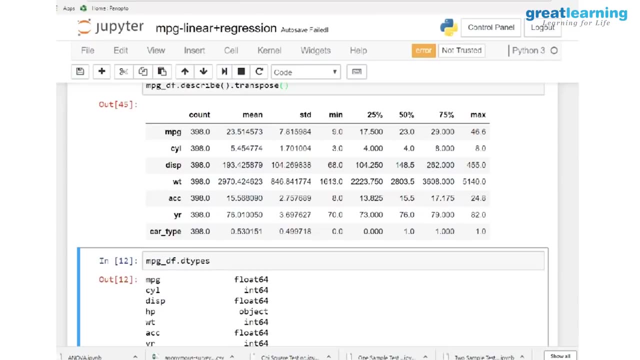 Q3 minus Q1 is called interquartile range. Any data point which lies 1.5 times IQR on this side or that side. they are generally candidates for outliers. So this is clearly telling us in the displacement column we have outliers. 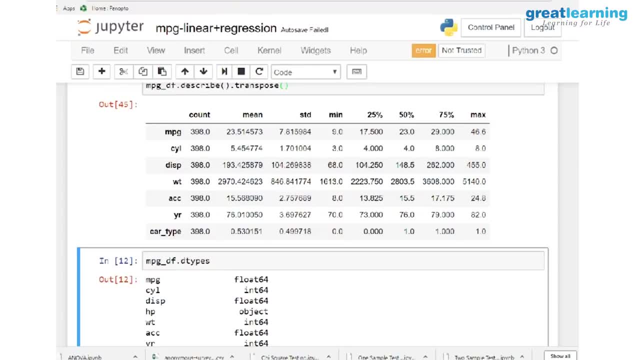 Similar analysis you have to do for weight and acceleration. You describe statements and you see any columns missing there which you are expecting there to be there. That is an indication of data pollution. When any non-numeric character gets into a numeric character and you do describe on it, it will not reflect. 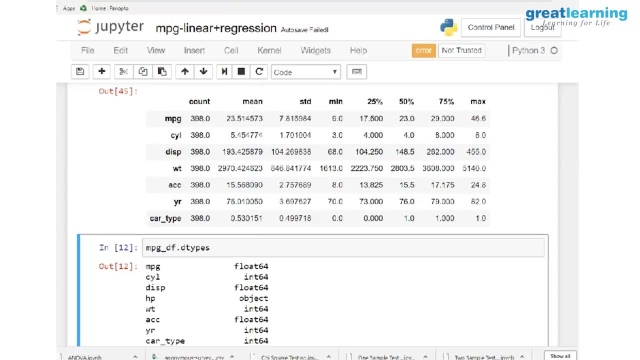 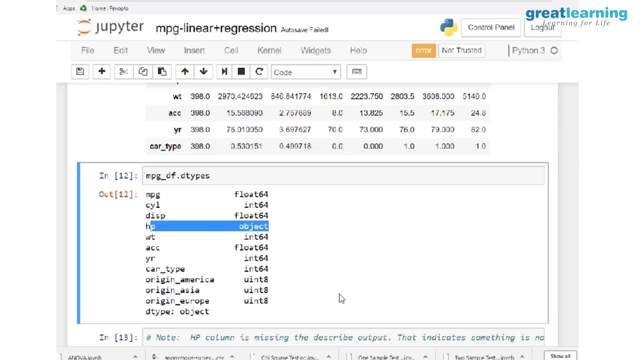 We can handle this, which is what you have done down the line. Come here, Look at these data types. When I saw that missing HP, I went and saw data types. HP is object data type. I thought it was numeric. It is not numeric. 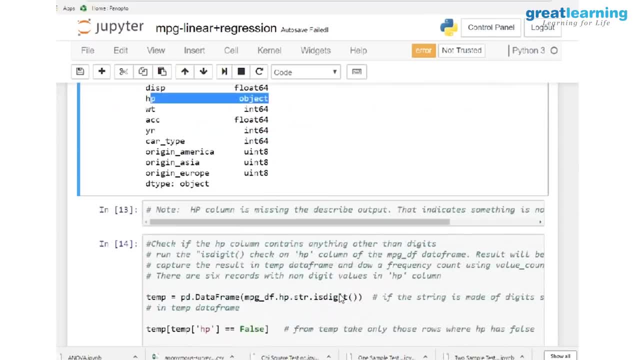 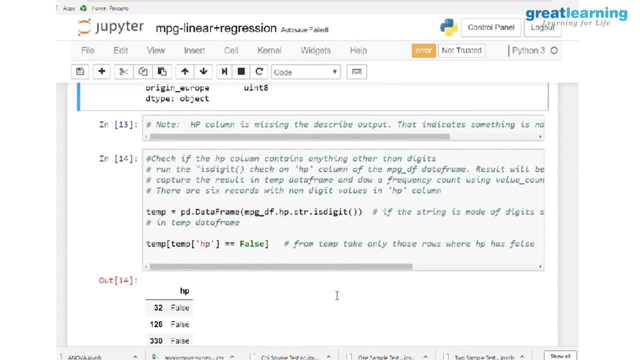 Object means string data types. Then you further explore: why is this object data type? Why the Pandas convert into object, Why not into numeric? For that, what you do is: I am applying. look at this. I am applying a function called isDigit. 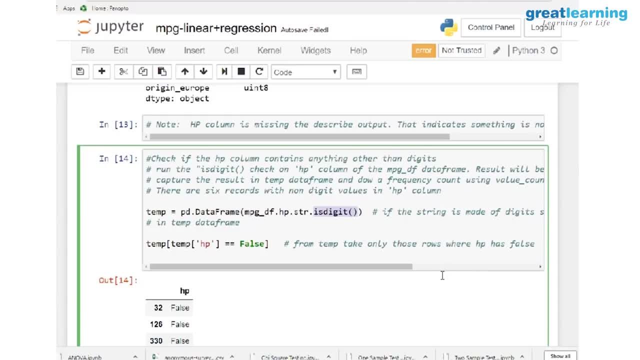 isDigit is a Boolean function. This function will return a true if it is a digit, false if it is not a digit. So this function I am running on this column called HP. If the HP column has numbers in it- 0 to 9, it will return as true. 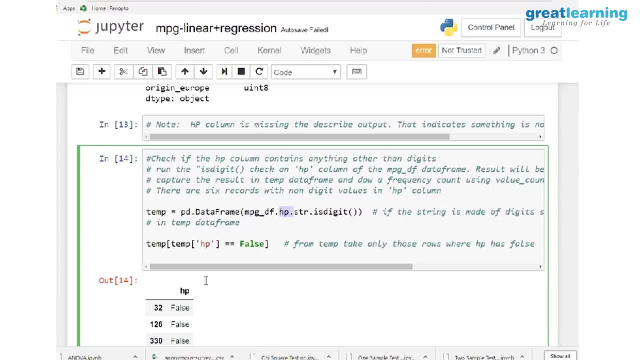 If its number is anything but 0 to 9, it will return a false. So this temp which you see here is nothing but all the records, as many records as you have in the sample, say 1000 records. Some of them will be true, some of them will be false. 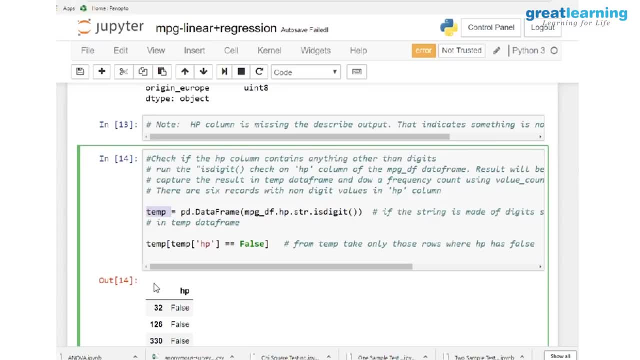 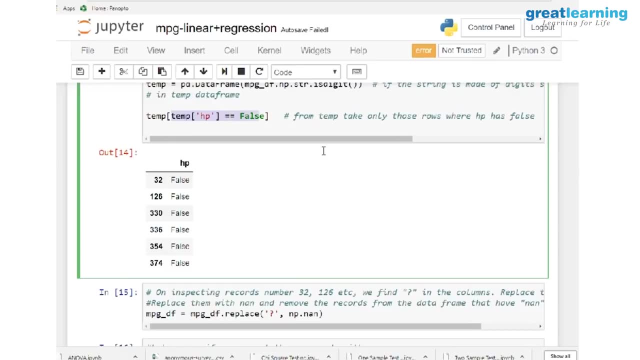 Those records which have a false. they are the ones which have a question mark in the HP column. So when you do that and then I say from temp, the HP column, print out all those columns which are false, it gives me the record numbers which are false. 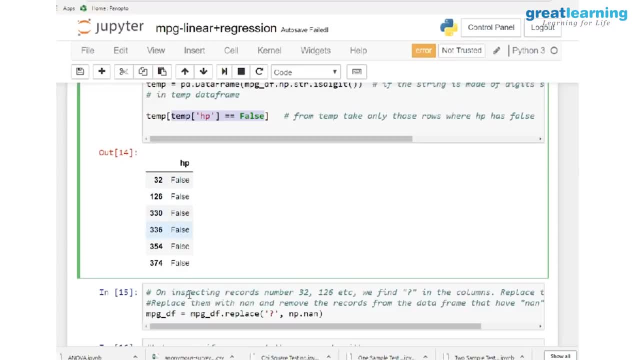 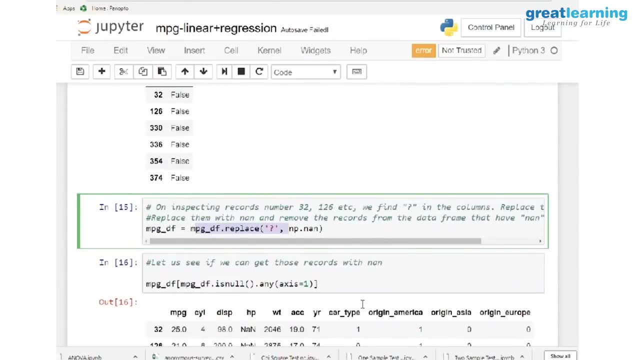 Then I go and explore this record- number 32,, 126 and all in the CSV file- I notice they have a question mark. Because they have a question mark, what I do here is I replace all the question marks with numerical Python NAN. 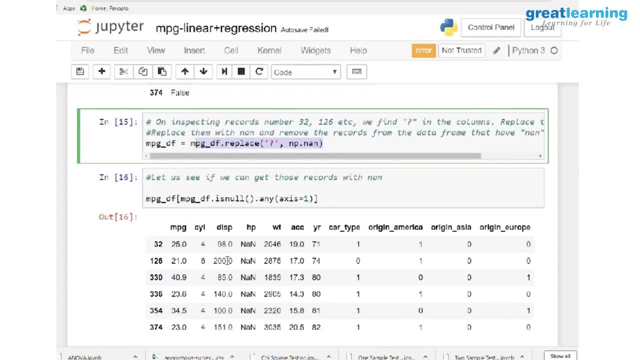 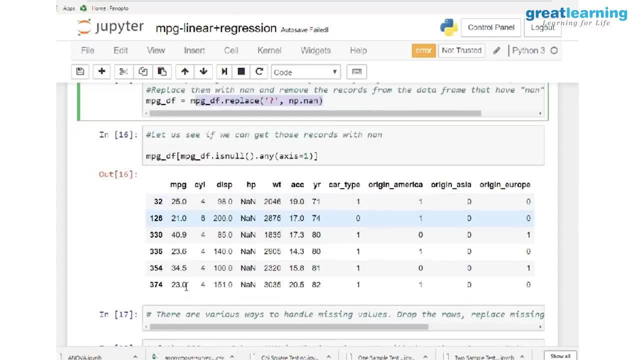 NAN means not a number, it is a null. Again, on mpgdf, I fire isnull command. get me all the records which have null values in them, just to make sure that only these records are null. See, these are the same records which you found here. 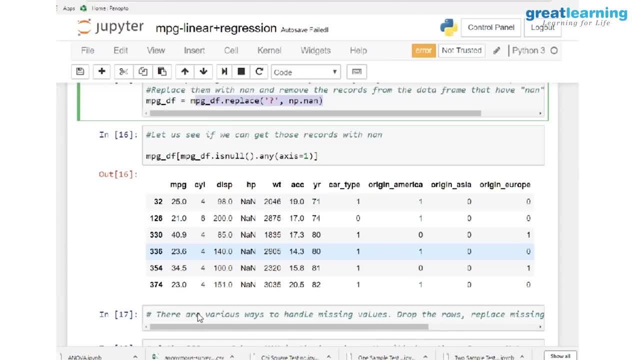 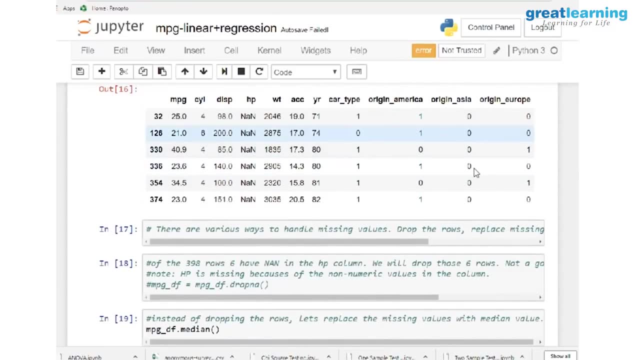 So I am convinced that there are no question marks anywhere else, no nulls anywhere else, So only these records are culprit. So what I do here is I go and replace all these missing values, the question marks, with median of this column. 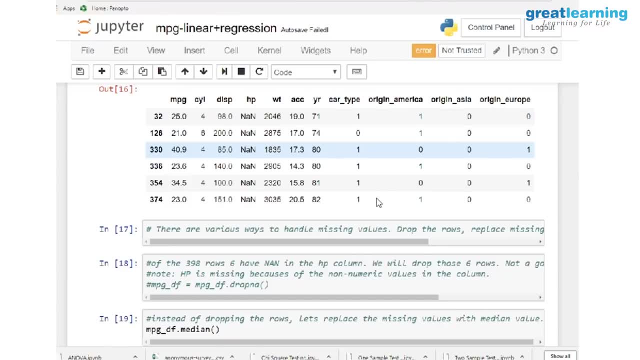 Why median? Why not mean? You can ask me those questions. I don't replace with mean because mean gets easily impacted by outliers. They are not reliable metrics, so the best option is median. However, in real projects, when you do these things, 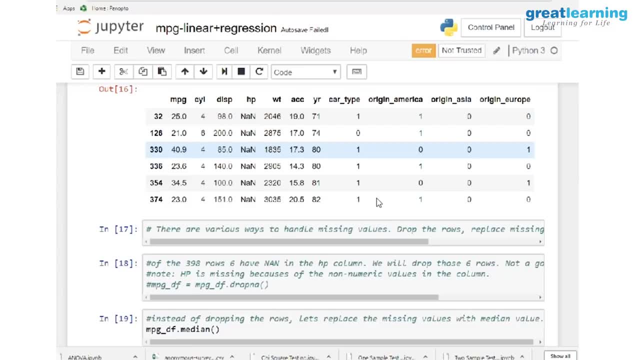 you have to take a call. you have to think twice before you use any strategy of replacing values. By replacing these missing values with median, I might be introducing a bias in my dataset. If there is a big chunk of missing values, there are options. 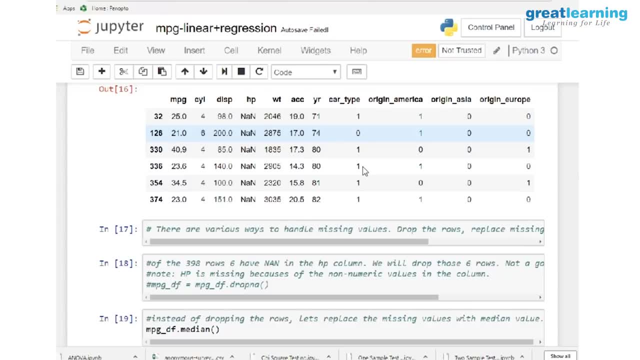 Do you think the column is worth it? Drop it If you think the missing values are not too many. this is where I like R In R. there is a package called mice. Nice name This package, mice package. it automatically builds submodels inside your datasets. 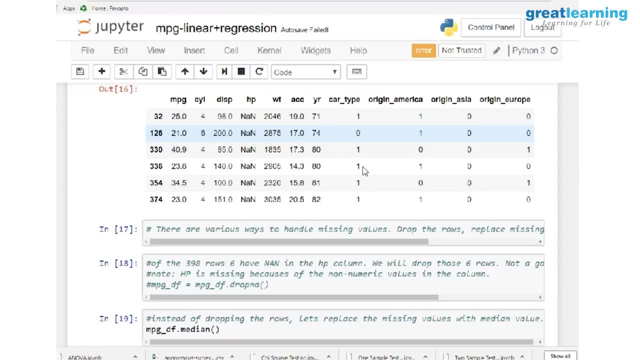 To try to predict the missing values in a column based on the values in the other columns. It's not available with the download of Anaconda, though it's available for pip install if you know how to do it, Okay, Mice package. 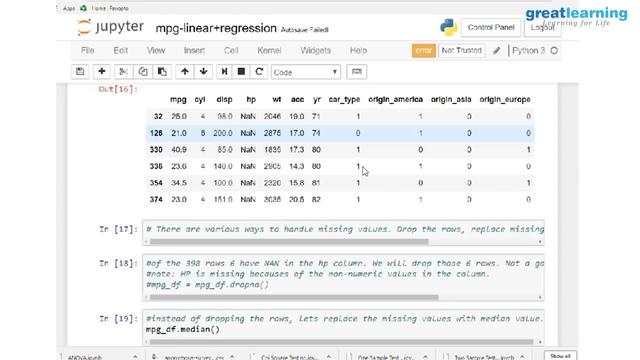 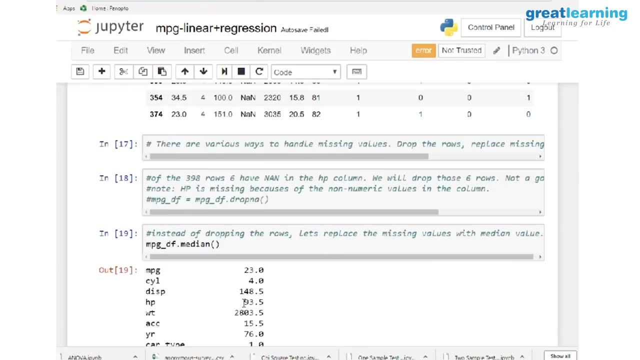 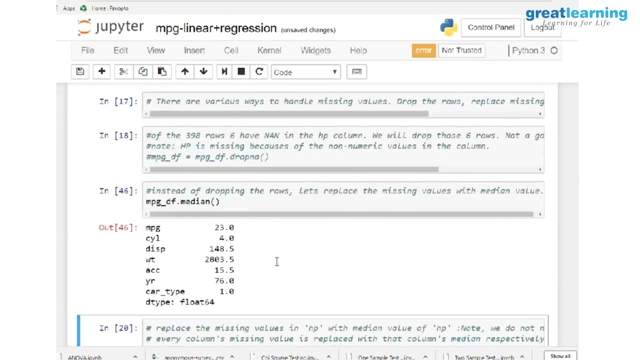 Otherwise, you build your own correlation between the dimensions and see if there is any dimension which predicts this dimension in which values are missing. Can I replace the missing values with predicted values? So I'm replacing, I'm doing mpg underscore median. Now how is it that it's able to give median for horsepower column? 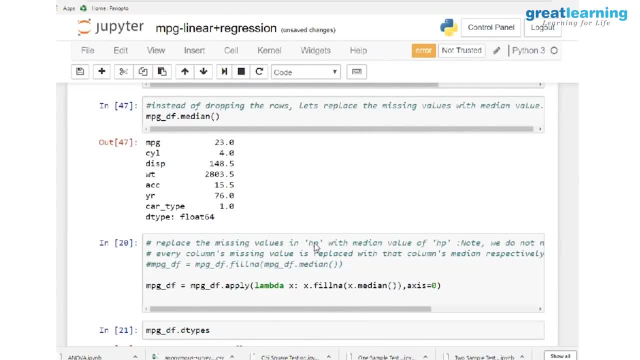 The other advantage of replacing with median is median is not an arithmetic average, So that particular column doesn't have to be numerical column. Median is physical central point, So you don't need to calculate anything. So that's why it doesn't have to be numerical column. 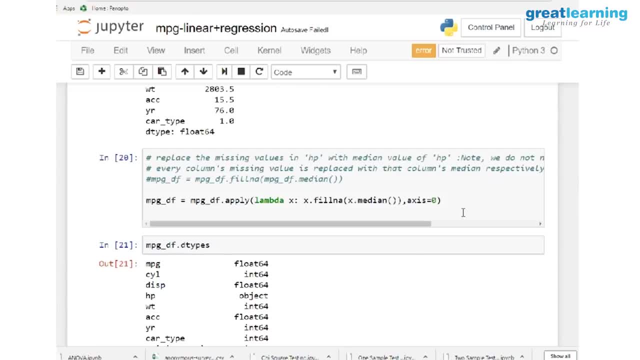 Now here. what I'm doing here is I've written a small function. In this function, what I'm doing is I'm replacing all those NAs with the medians. What I'm doing here is I'm going column-wise. 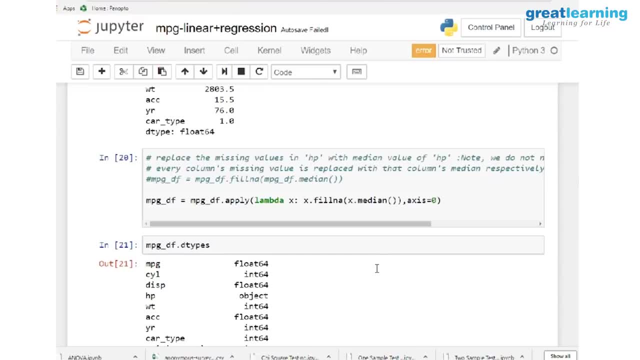 The X represents a column. here In the column. whenever you find any NA, replace it with the median of that column. So it goes column-wise in your data frame. If in any column it finds an NA which is not there, except for in horsepower column. 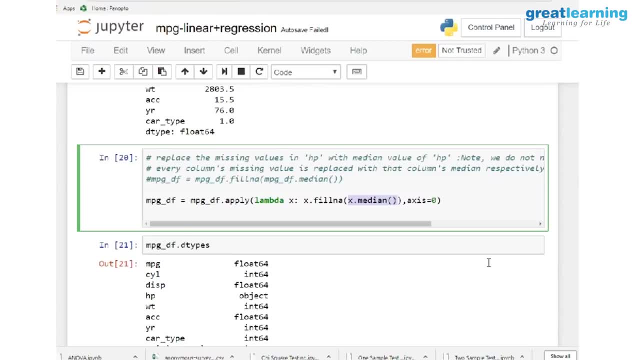 in horsepower column it replaces the NA with horsepower median. That is what this line does And this is called lambda function, where you define the function based on your needs And apply is like a for next loop. It will go column by column, for column 1 to column N. 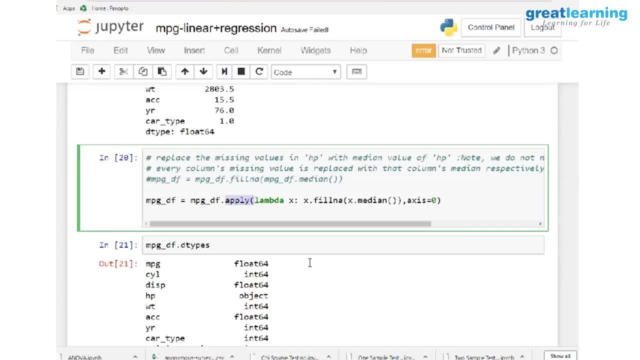 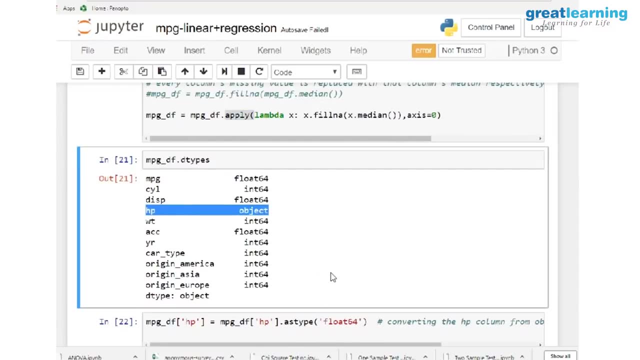 Look for NA in the column. If NA is found, replace the median of the column. When I do that, then my horsepower is filled up, but it's still object. So I convert it into a float type here. So what I'm doing here is: 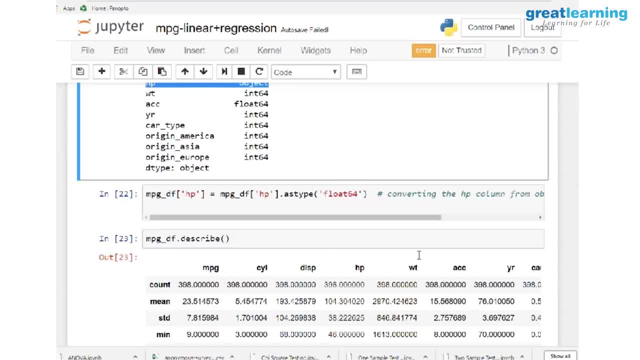 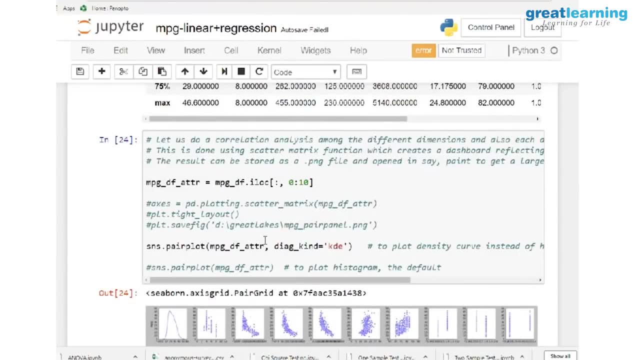 I'm changing this horsepower type. I'm changing the type from object to float. Once I've done that, now, if I do describe, you'll see horsepower there. At this point, what I'm doing is from the data frame, all the rows. 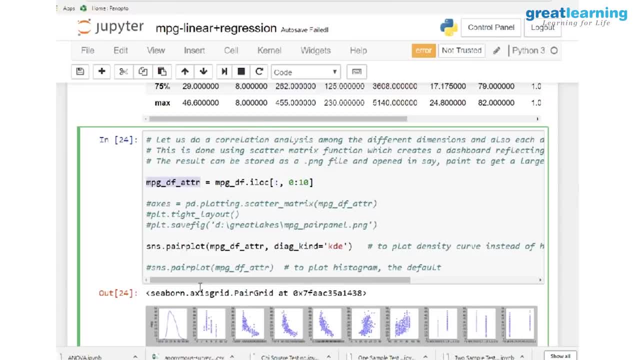 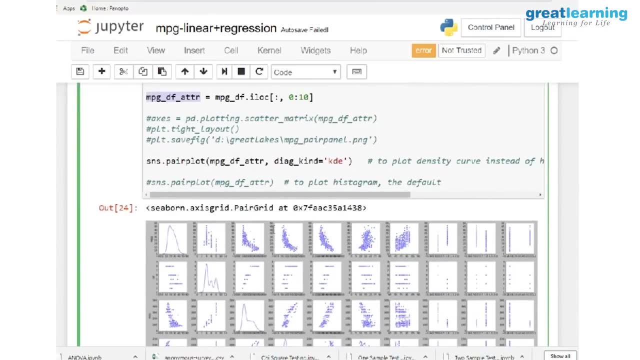 first 10 columns. I'm storing them into a separate data frame called attributes. These are my independent variables On this. I'm running a pair plot. Don't run this pair plot now. It'll take long time, but it's going to do 10 x 10, 100 pair plots. 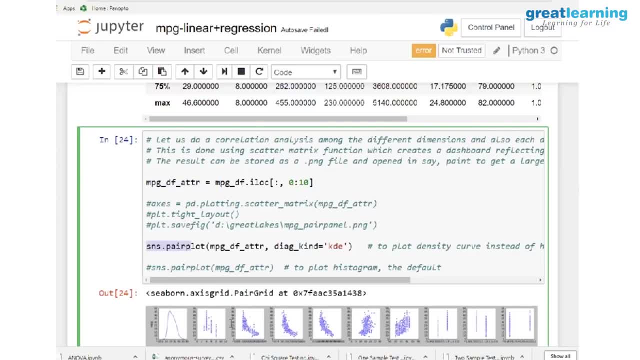 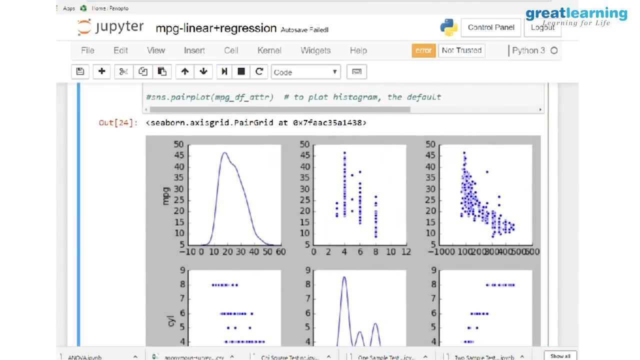 On this I'm doing SNS pair plot. SNS is a seaborn library And the pair plot gives you this. Are you able to see this? Double click on this. this will expand. Double click on it, it'll expand. 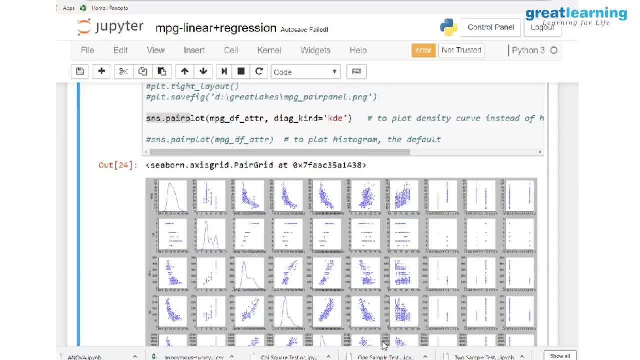 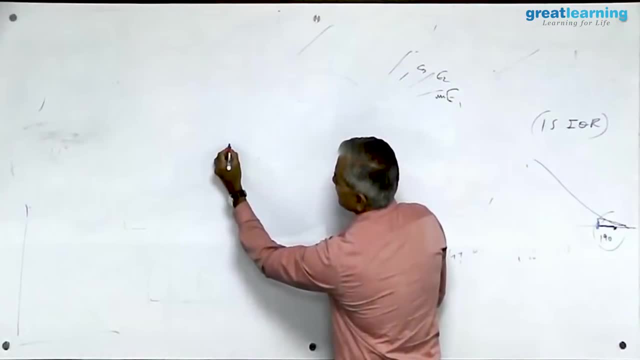 Now this pair panel. how do you interpret this? You have the 10 columns. All of you know how to interpret pair panels. You have 10 columns. Can you quickly tell me what those columns are? MPG. next column is: 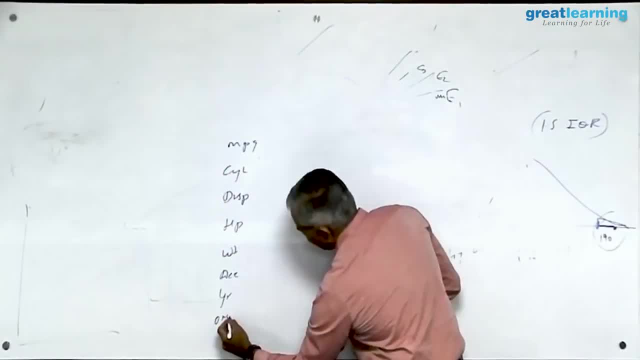 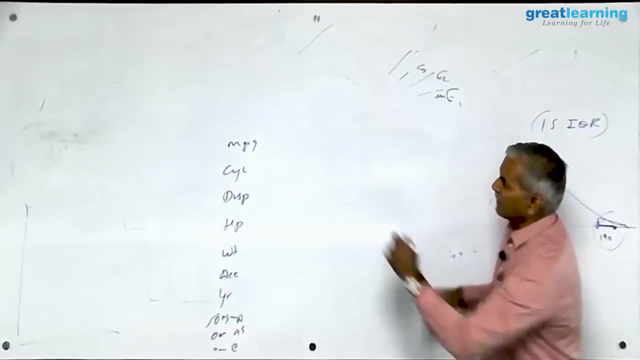 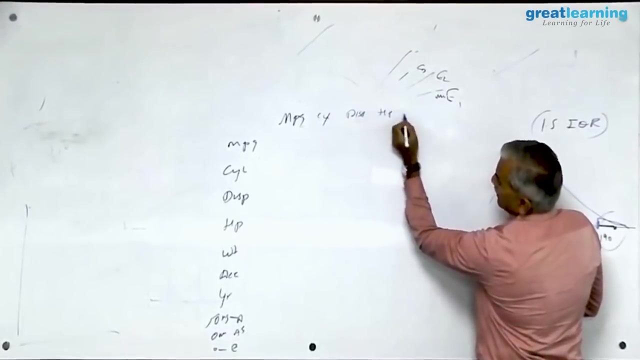 Cylinders, next Displacement, next Weight. All right, This part origin America, origin Asia, origin Europe. Same columns, keeping them on the top, also MPG. you have cylinders, you have displacement, you have horsepower, you have weight, you have acceleration, you have year. 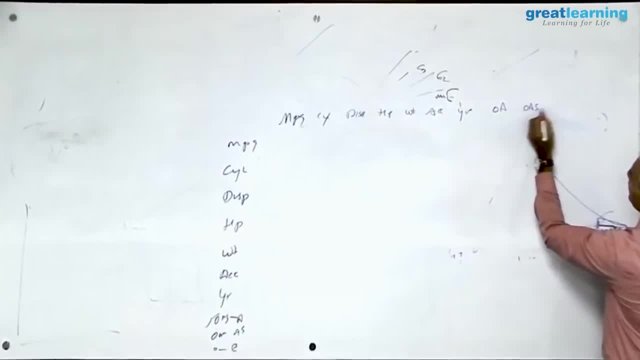 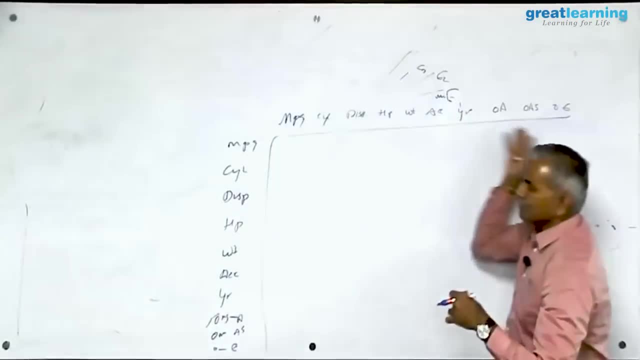 Then we have origin America, origin Asia and origin Europe Matrix. it's a square matrix. We call it a square matrix. As many rows, as many columns. What you're seeing here is how MPG and MPG is related, which is nonsense. 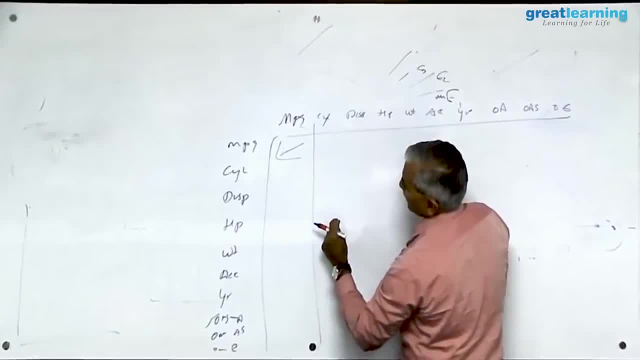 If I do a scatter plot between them, I'll get a straight line. So, instead of giving you a scatter plot, what I've done is I've used KDE. KDE stands for density plot, Diagonal kind is density plot. It's giving you a density plot. 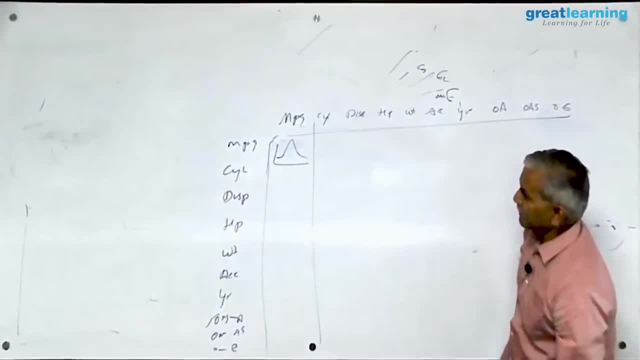 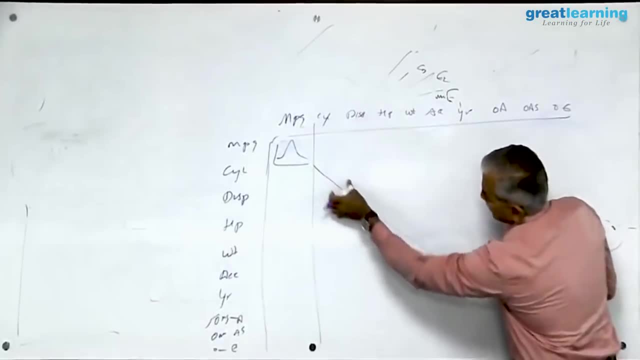 The beauty of the density plot is it's telling you a lot of things. Then, MPG versus cylinder, So you go diagonally. All the diagonals will be density plots. What you see on the top will be mirror image of what you see on the bottom. 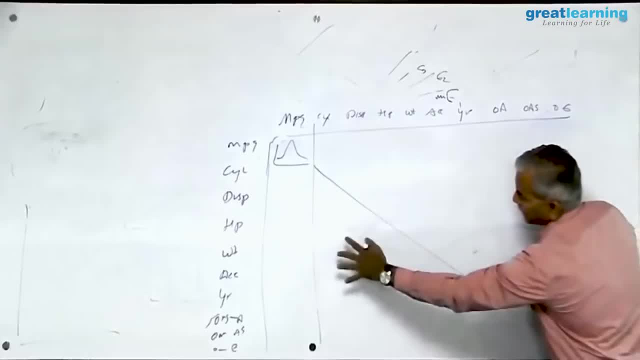 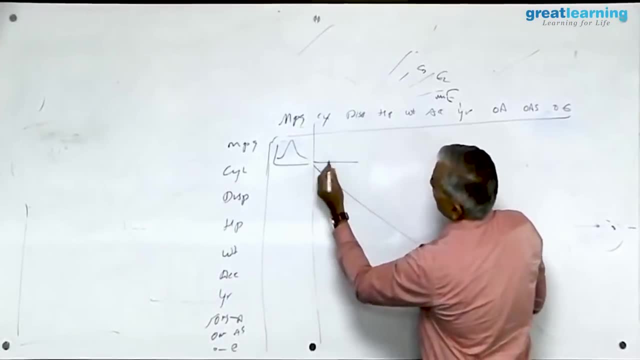 Either you look at the bottom or you look at the top, So you can take only one half. How is MPG related to cylinder? You see over there. So lower the cylinder, more the MPG, Increase in cylinder, fall in the MPG. 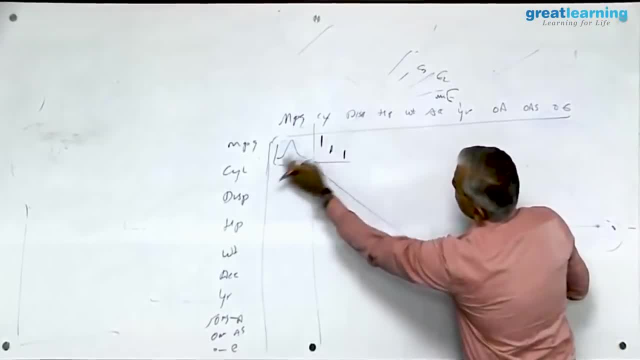 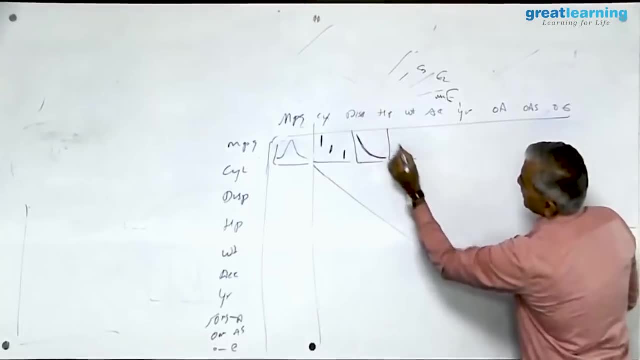 That's what you're seeing, the trend over there. How is MPG related to displacement? You'll see a downward line negative relationship. Similarly, you'll see a negative relationship. Weight also: you'll see a negative relationship. Acceleration also should be negative. 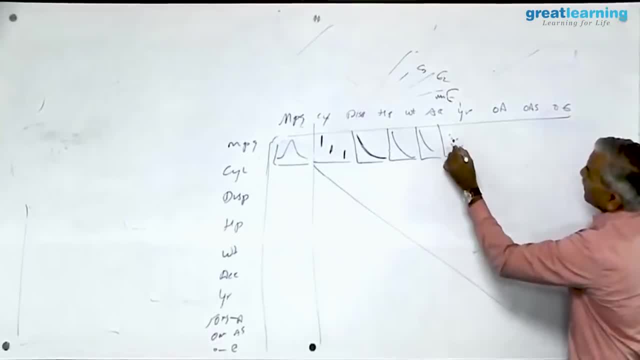 Acceleration: no correlation Year. you'll see as the year increases. I think it's positive correlation. This is year of manufacture. As the year of manufacture increases, that means the age of the car decreases, your mileage goes up. The brand new cars give higher mileage than others. 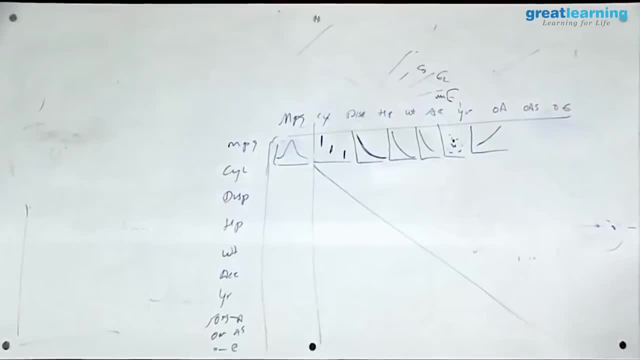 Origin America and Asia and on. You'll see them as lines. What is these two lines here? Origin America, origin Asia and origin Europe. You'll see two lines here. Origin America: one means America. zero means other cars. In case of Asia, one means Asian cars, zero means other cars. 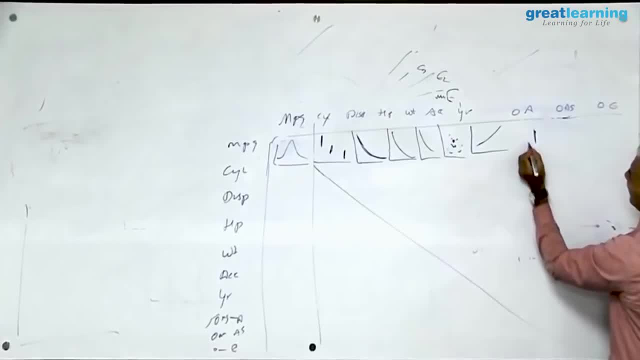 So the one here you'll see on the lower side and others on the higher side. American cars generally give lower mileage. They're fuel guzzlers. Asian cars, you'll see that they give higher mileage and others will be slightly lower, Because others include European and American cars. 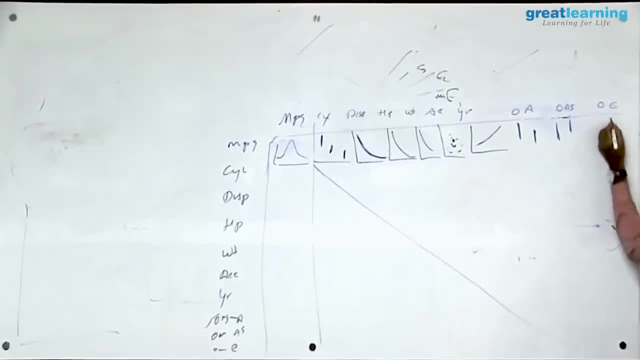 Similarly, origin Europe, you'll see higher mileage and the other categories, Asia, and this will be slightly pulled down. You'll see this kind of trend. Is that correct? Yeah, correct, That's it. So, of all these dimensions, this particular low. 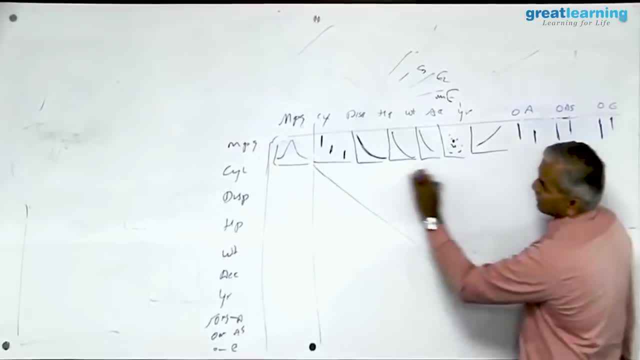 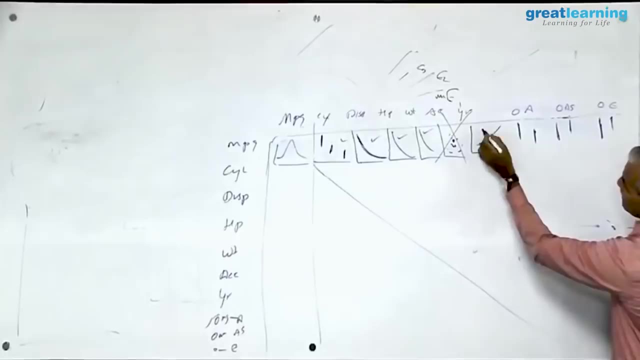 it tells you to identify which dimensions should you use to predict MPG. Obviously, acceleration column is not a good choice. These columns, they have some kind of relationship with MPG. Even cylinder has a relationship with MPG. Even this year can be considered for MPG. 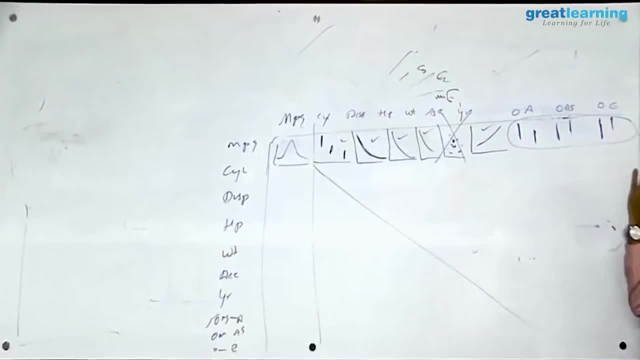 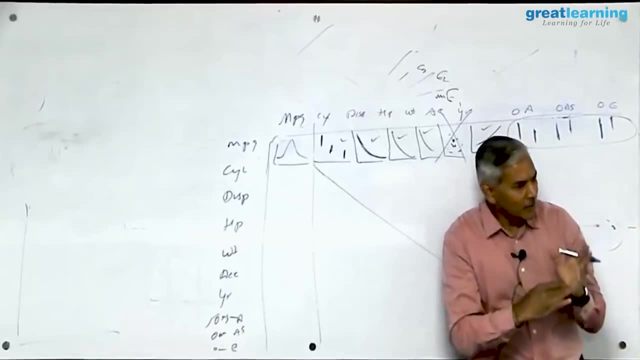 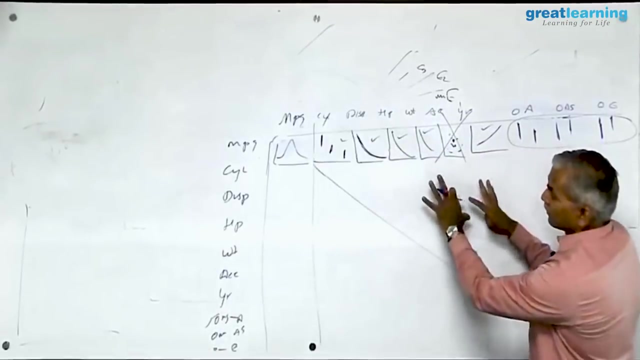 These three are suspicious because they are significant to overlap in the distributions. So pair panel is one of those tools that you will use in all our model building exercise to decide which attributes are important predictors of the target, One of the very important tools. The other thing that you should focus on is the diagonals. 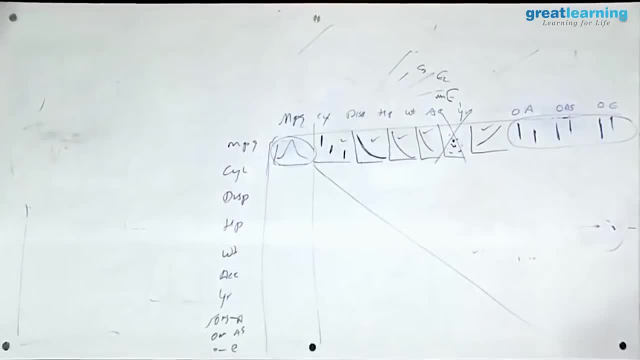 Look at the diagonals. Look at this one. This is: you see three gaussians there. You see three gaussians there And you come down the diagonal. The next diagonal is displacement. In displacement also, you see three gaussians, but those gaussians are not very clearly visible. 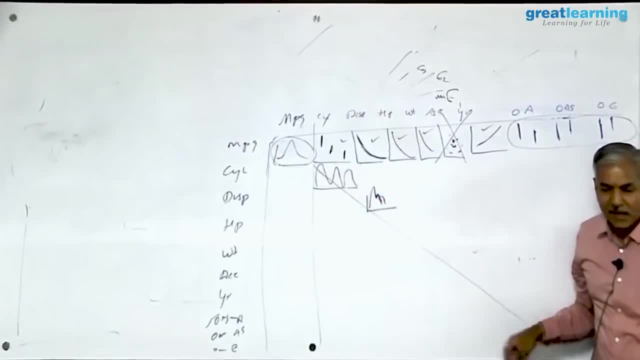 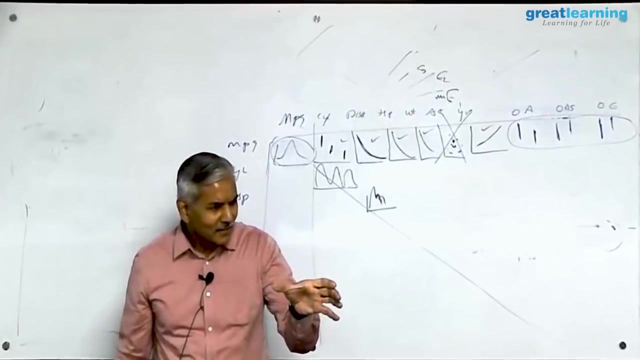 Always look at the density plots And in density plots if you see multiple gaussians here, that means you are in trouble. What are we doing? What model are we building? Do you think mileage of all these cars, whether they are large cars or small cars? 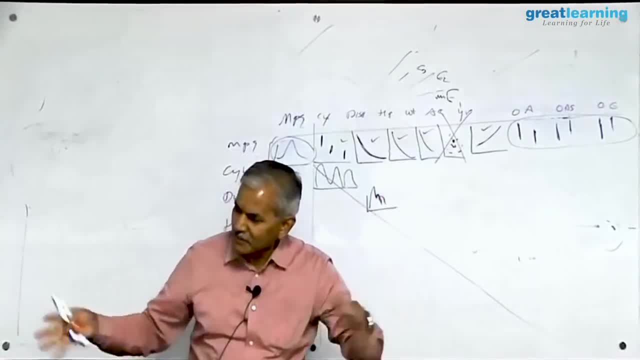 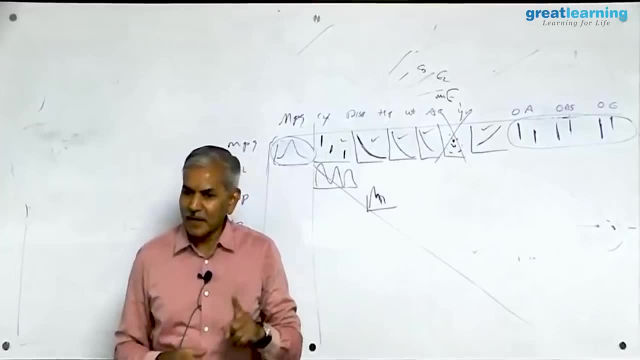 do you think the mileage of these cars? do you think they have the same attributes, Do you think they enjoy the same characteristics? Then do you think we should be building one single model to predict the mileage of whether it is a Maruti 800 or Toyota SUV? 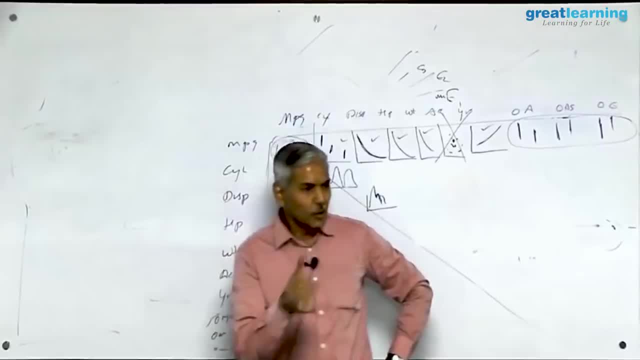 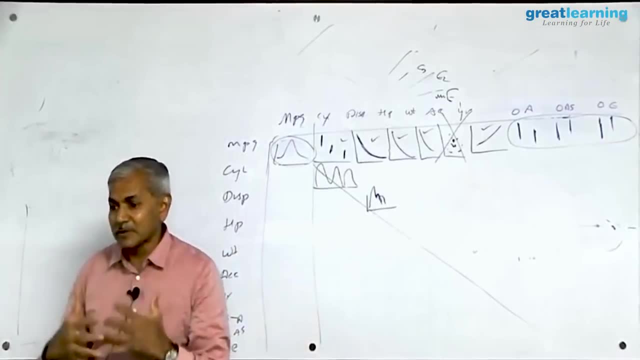 But that is what we are doing. So whenever you are building models, look at your data set. In the data set, if there is any evidence of mix up of gaussians, this is what we call mixing up of gaussians. Gaussians, when they come, they come from different processes. 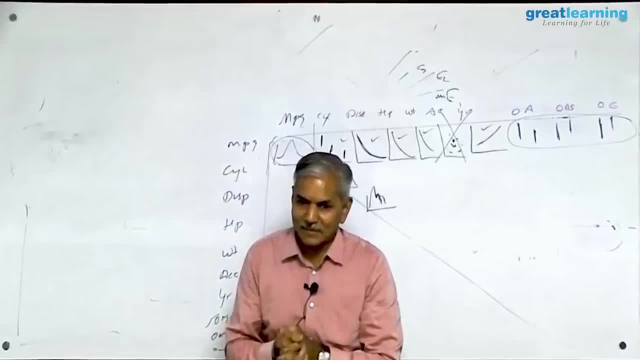 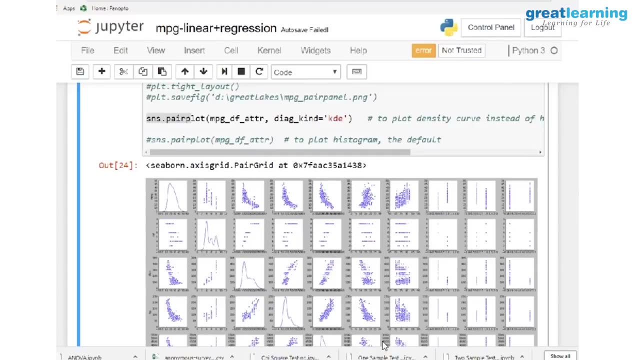 You are building one single model to represent all the processes, which could be a mistake. When you do a scatter plot between MPG and MPG, you will get a straight line, So that is a useless analysis. So, instead of getting a scatter plot, 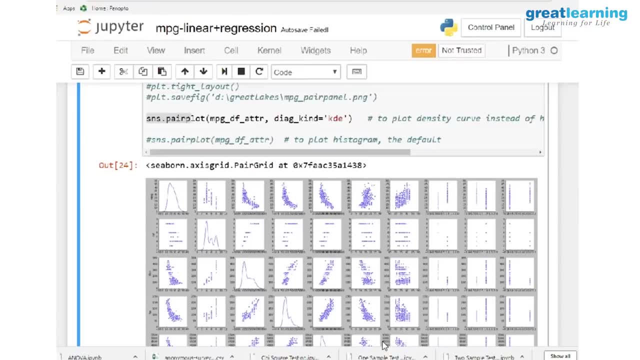 I ask you to replace the density. How is the data distributed on that dimension? So this is a distribution of data on MPG dimension. It is not a scatter plot of MPG versus MPG. It is not telling you anything about the relation. So this is telling you how data is distributed on MPG. 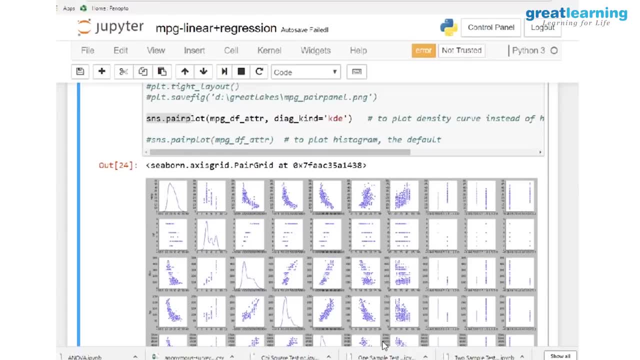 This y-axis is meaningless. Now, whenever you have your data like this, where the dimensions are clearly telling you you have multi-gaussians there, you need to be careful. Do you think it is right to build one single model for all these gaussians put together? 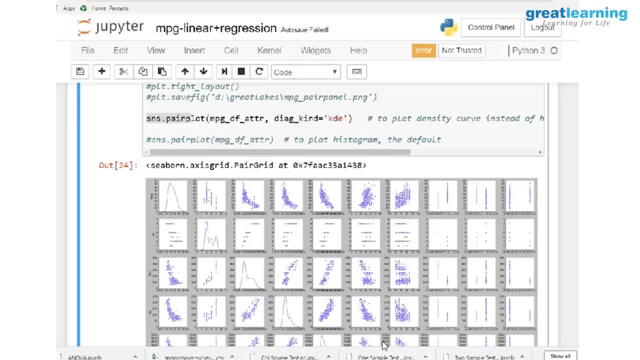 Or should you segregate these gaussians into different data files and build models separately on them? So obviously, when I build a model to predict mileage, I will build a separate model for small curves. I will build a separate model for large curves. That is the advantage of doing pair passing. 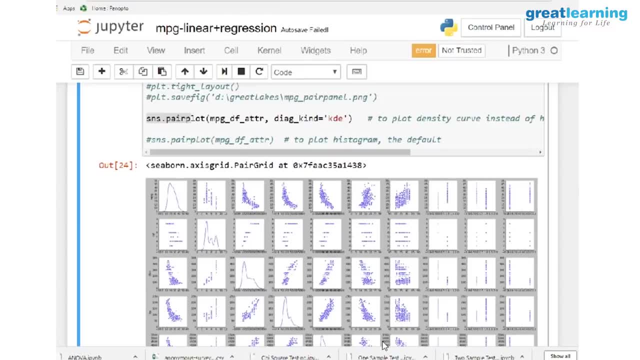 So this is a very important tool in all the algorithms in supervised learning. How the data is distributed on your dimensions will come out clearly on this. Based on this, based on this analysis, you will decide: do you think linear model is good or should I make it quadratic model? 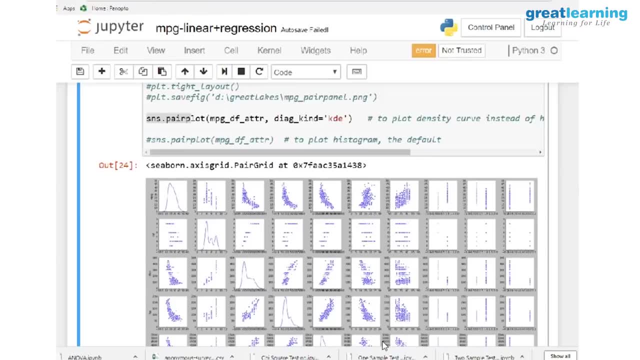 That is what we do in unsupervised learning. We always start with unsupervised learning. In unsupervised learning, we see multi-gaussians there. Clusters, Clusters are gaussians. Then I go and investigate those clusters. 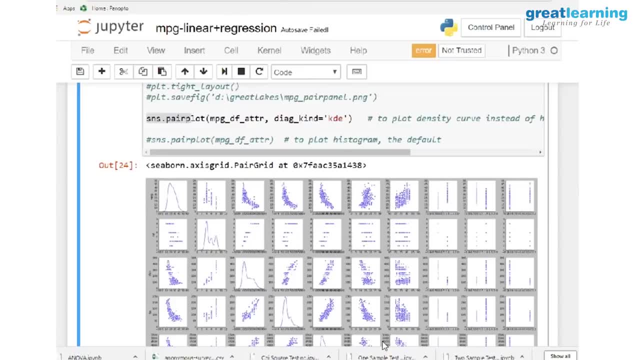 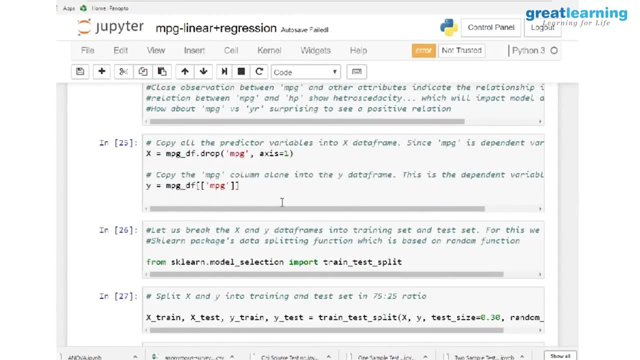 Why are there so many clusters? What is this cluster about? What is this cluster about? I give meaning to them. What I am doing here is I am taking all the columns except mpg column and keeping them in x. x stands for independent variables. 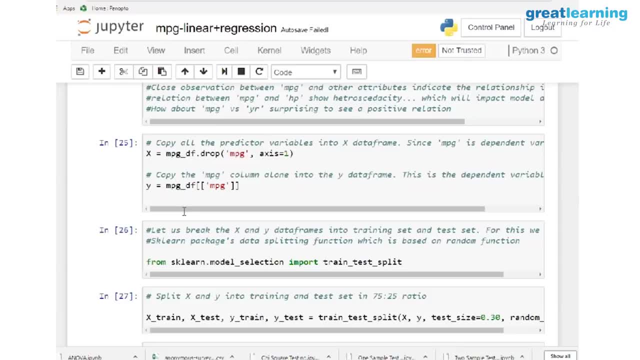 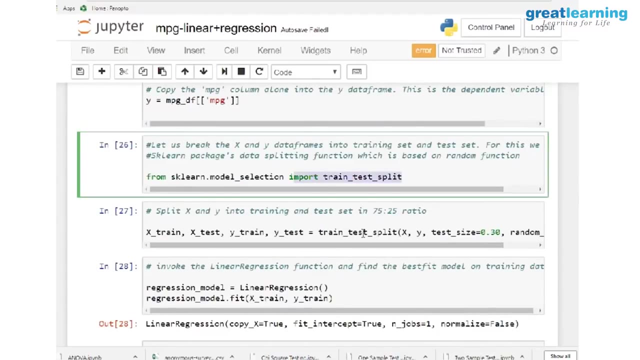 It is a practice to represent independent variables as capital X and the dependent variable, which is mpg, in small y. It is a practice, You do not have to do it, But this is general practice. And then here I am importing a function. This is a function from scikit-learn called train test split. 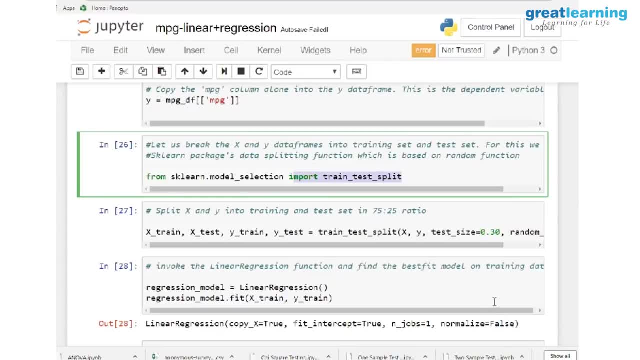 What this function does is. this function takes as input your x and your y and randomly breaks this into training set, test set. Doing so. here you are given the test size as 30, which means 70-30 ratio, So it will randomly pick up data and put into training set. 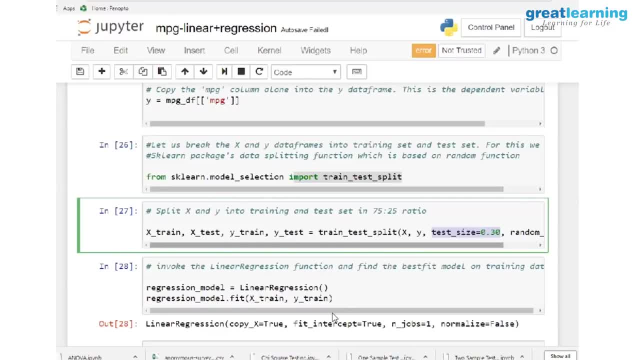 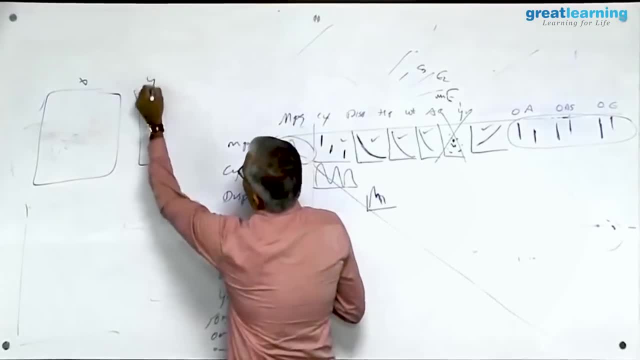 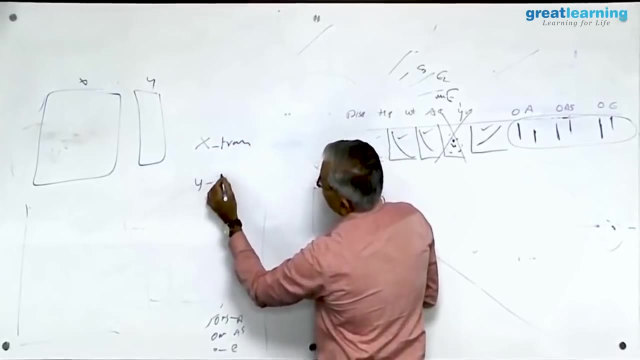 and randomly pick up data and put into test set and the ratio it will maintain is 70-30.. So this is my original data frame, This is my x and this is my y. This I am breaking into x underscore train, y underscore train. 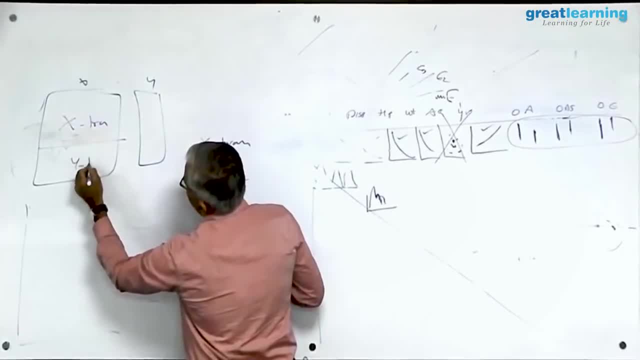 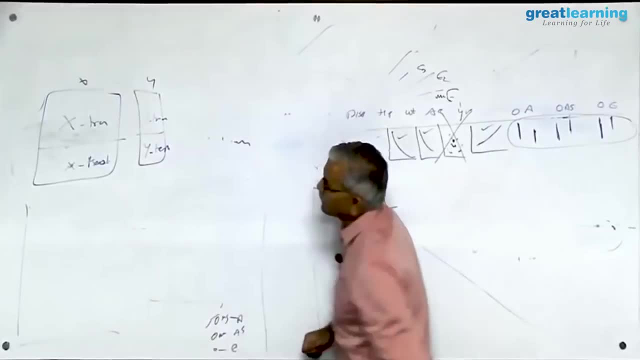 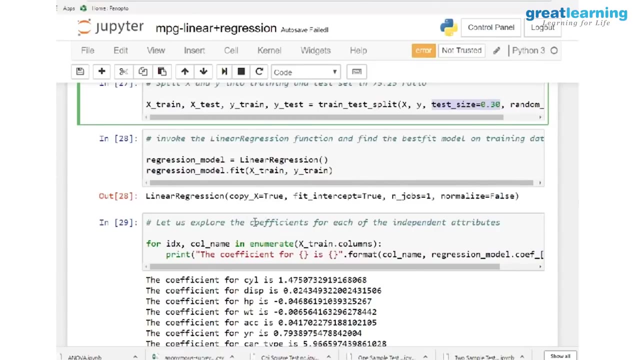 So this is my x train, y underscore train and this is y underscore train and this is y underscore test. This is what I am doing with the original data And down this line I am here instantiating the linear regression model. And to the linear regression model. 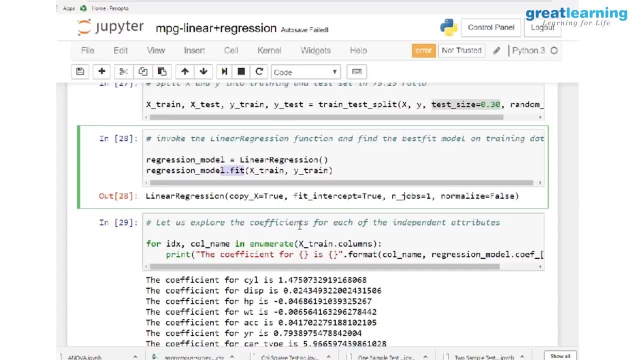 I am given the fit function. Remember I told you, every algorithm has a fit function. To the fit function. I am feeding the independent variable training set Dependent variable training set. This is what we call labels. At this point the gradient descent algorithm will come into play. 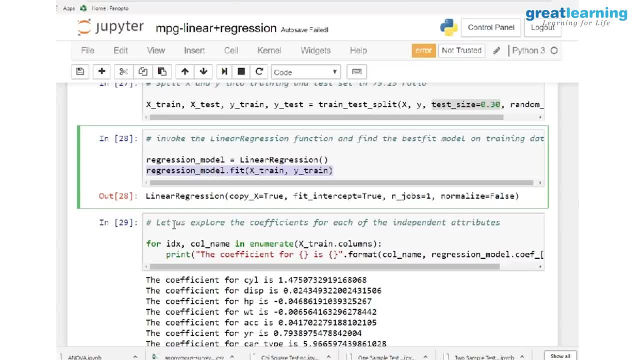 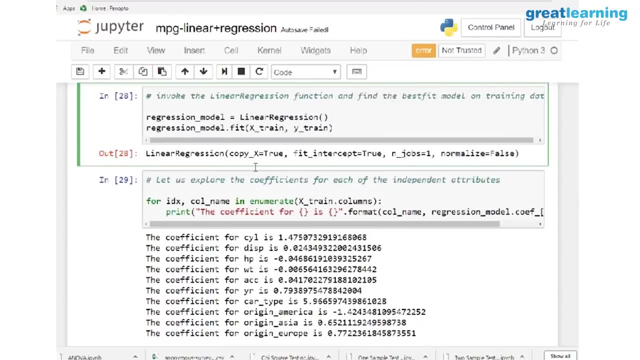 It will find the best surface for you, The surface which gives you least sum of squared errors. All those things will happen at this point. Once I found this point, then, what I do here is this object which you call regression model, This object you have created now. 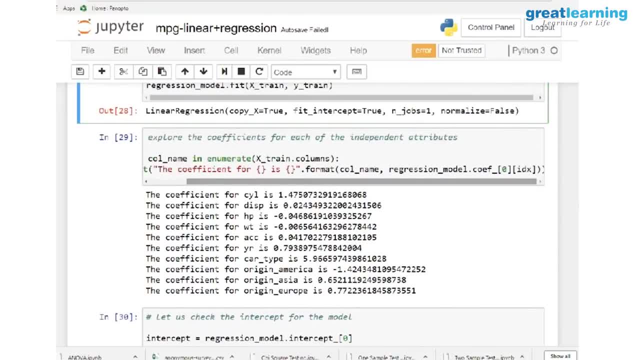 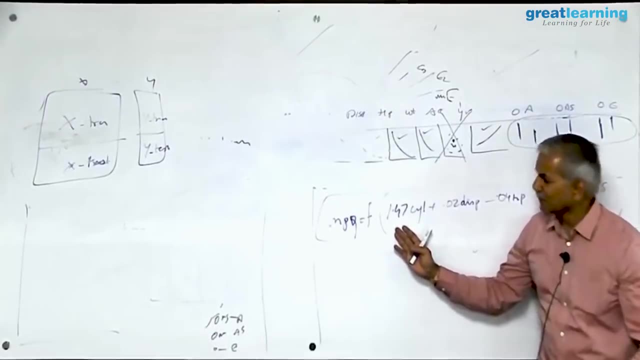 In this object. this algorithm stores all the coefficients in a particular array. So I am using a function called get coefficients. It is printing the coefficients for all the dimensions here. Looks suspicious. Actually, with increase in cylinder it should go down. That clearly tells you data is in problem. 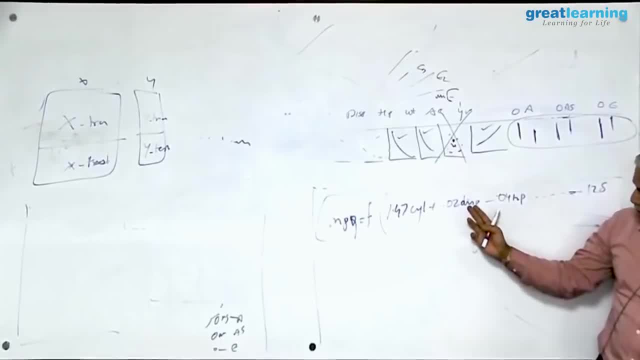 Every unit increase in displacement increases your MPG by 0.02.. Every one unit increase in horsepower decreases your mileage by 0.04.. That is what this equation is telling you. When all things are zeros, your miles per gallon is minus 128. 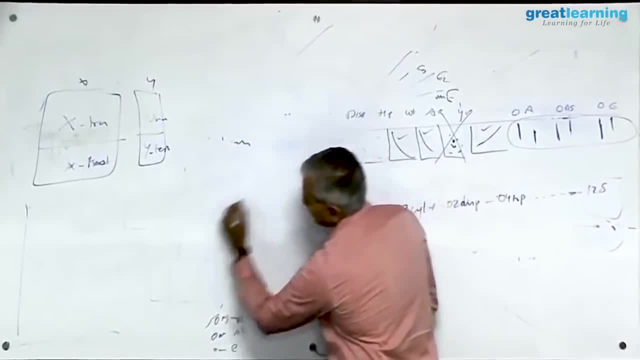 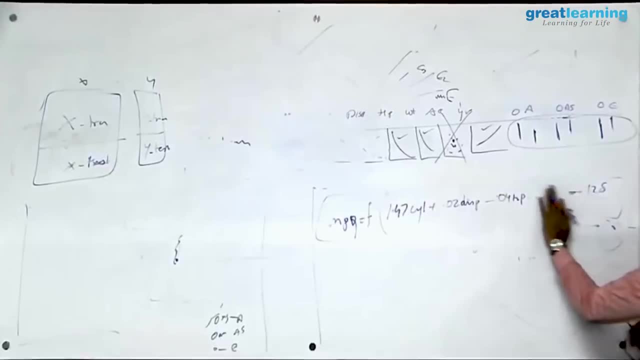 That is what intercept tells you. What is an intercept? Intercept is when x is 0,. what is this value of y? What this is telling you is when everything is 0, your MPG is minus 128. Now, what I am doing here is: 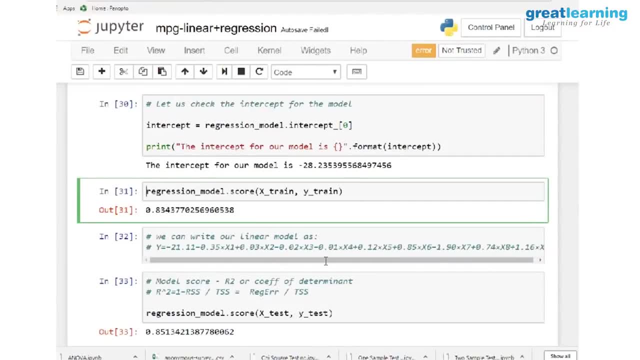 this model. this model, I am running on the training set itself to find out what is the accuracy in the training set. It is giving me accuracy of 83%. This 83% is your coefficient determinant, R squared. When I run this on my test data. 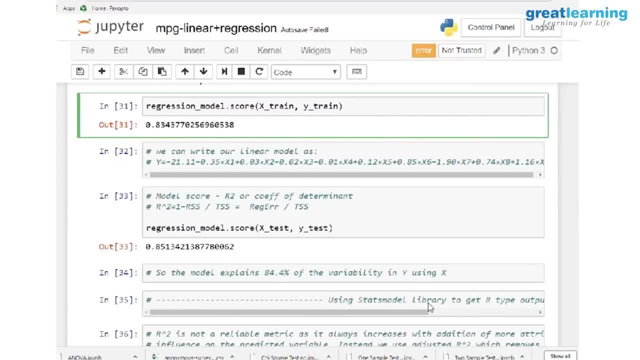 when I run it on my test data. when I do score on the test data, it is giving me 0.85.. 0.85.. This is just a coincidence. Now, what you should be doing is- and I am going to stop with this- 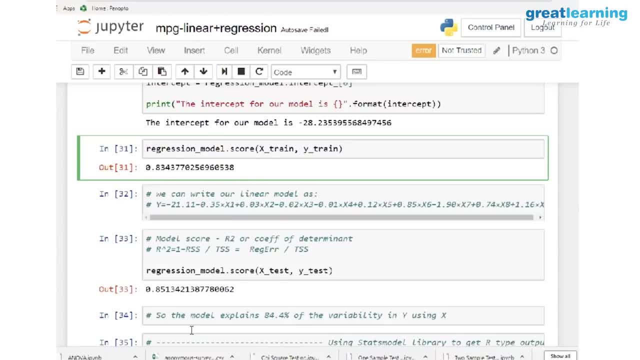 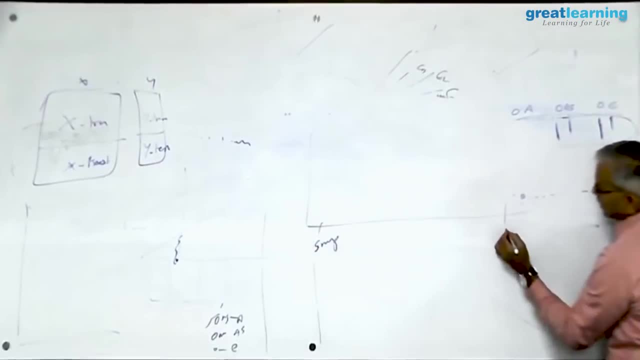 I will not go beyond this. It will be information overload. Whenever you build models, I told you, start with simple models, Simple to complex. How do you complicate models? I will tell you later. Always do your testing, both on training set.